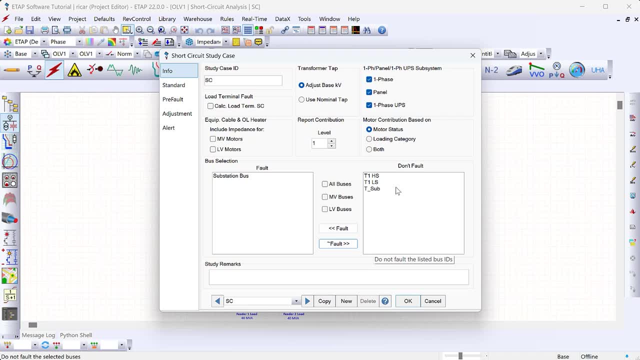 run short circuit. ETAP is not going to fault these buses that I have over here on the right. That's sometimes beneficial if you have a very large model with many, many buses. When you run the short circuit study it might take a little bit of time. 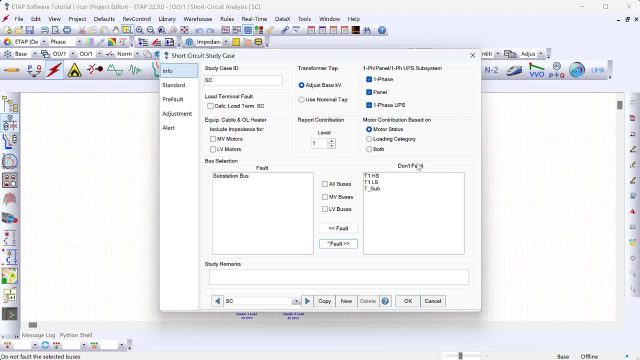 for ETAP to run the calculations, and so if you're only interested in some of the buses, then you can just put those over here and not worry about the rest, and that'll just help speed up the calculation for the fault currents. Now, in my case, we have a fairly simple model, so 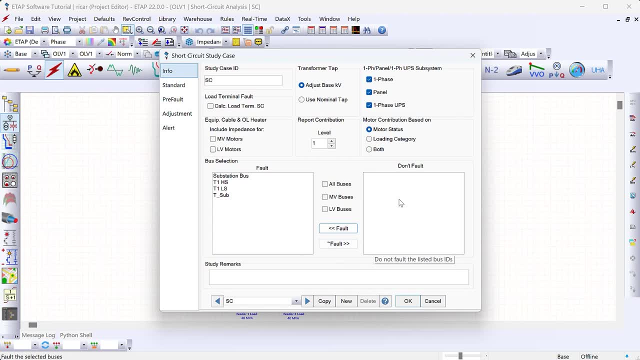 I'm going to fault every single bus in the system, so I'm going to move everything over here to the left. and here you have other options. for example, you can select the transformer tab for the short circuit study. So if you have a different tab position on your transformer, you can tell ETAP. 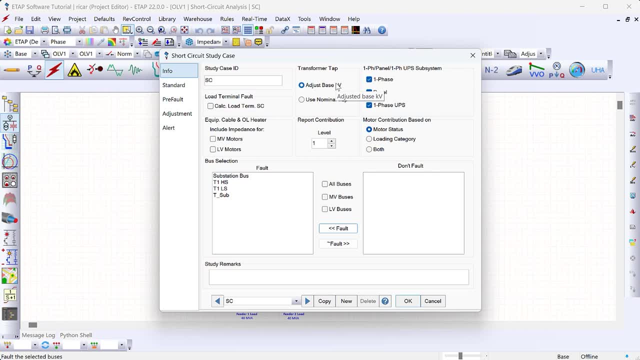 don't use that, use a nominal tab instead. or you can say: well, I use adjusted base kilovolt based on the tabs of the transformer. if you have a different type other than the nominal tab, You can also select over here the standard that is going to be used for running the short circuit. 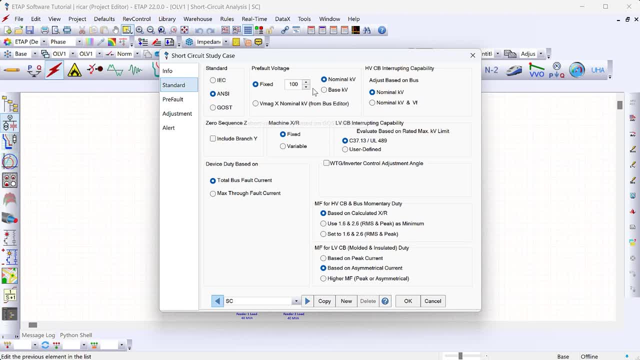 study. You can select IEC, you can select INC. you can also set the pre-fault voltage. So, for example, right now I have it to 100 percent of the nominal kV for the pre-fault voltage. So again, there's many options over here. typically you don't have to change this unless you want to. 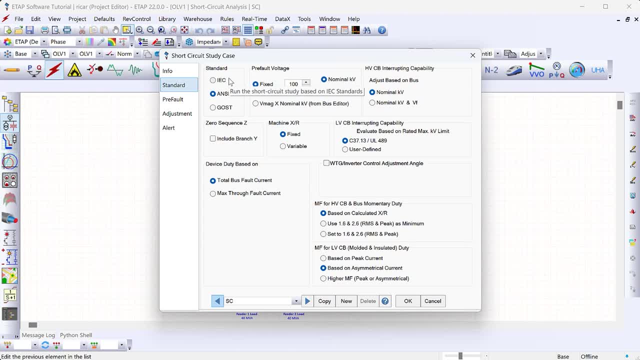 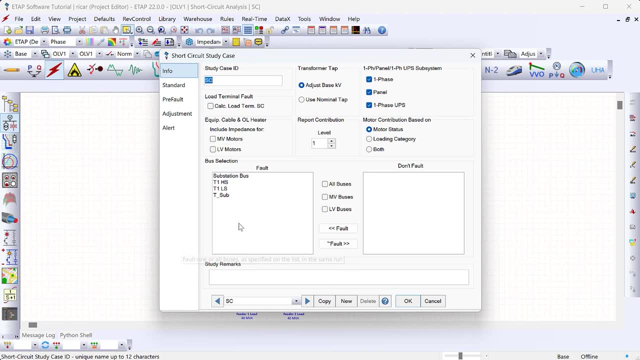 change something specific. for example, if you want to use the IEC standard instead of the ANSI standard for running your short circuit study. There's different options over here. I'm going to leave all of those at default. The main thing over here again is that I want to make sure that all 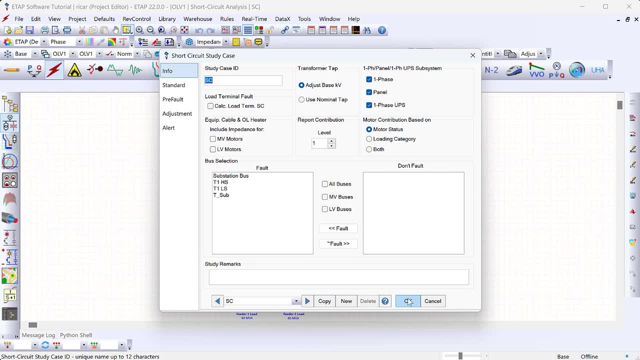 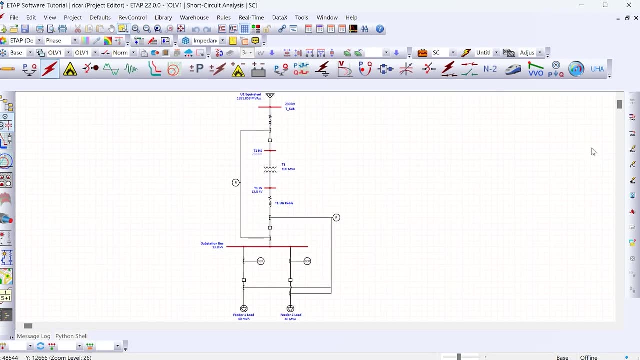 the buses in the system are faulted. So now I'm going to hit ok, and that's going to take us back to our model, and everything over here is blank because we haven't run the short circuit study yet. Now, the other thing that I want to show you over here is that you have these three options. 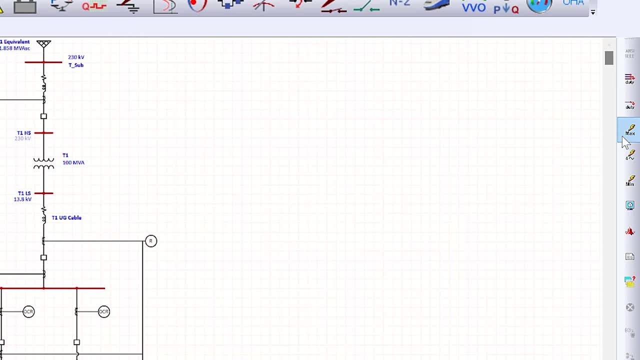 for running the actual short circuit. study Over here when you select maximum. what that does is it uses the sub-transient reactance for any synchronous generators that you might have in your system and it also accounts for contribution of motors during the first few cycles of a fault. 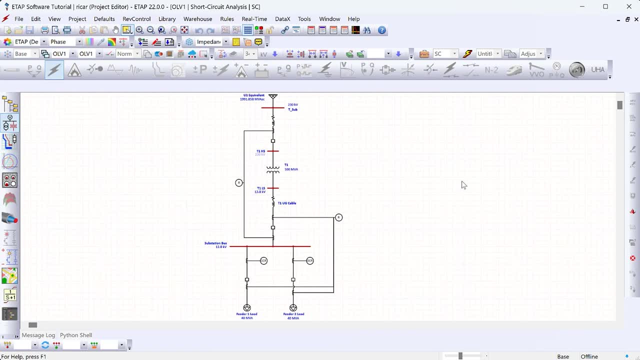 So, for example, in our model, if I click max now, ETAB is going to run the short circuit study and you can see that there's some contribution coming back from the motors to a fault on this bus. That's because for the first few cycles during a fault the motor is actually going to back feed. 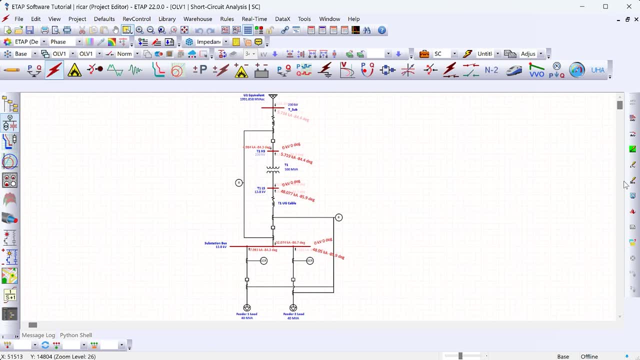 into the fault Now that is going to subside with time. so if you click over here, minimum what this does is it runs a 30 cycle short circuit, meaning it's going to tell you what default current levels are 30 cycles after default has happened, and that usually removes. 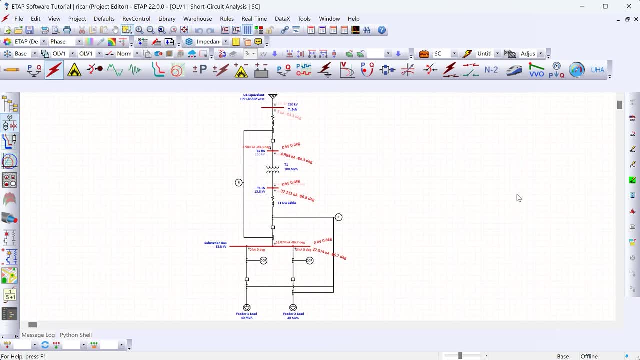 the contribution from any induction motors that you have in your system and also it uses the synchronous reactance for any synchronous generators that you might have in your system. So it's basically like a steady state fault, current level. after all, the transients have kind of decayed and you have a steady state fault, So just something to keep in mind, of course. 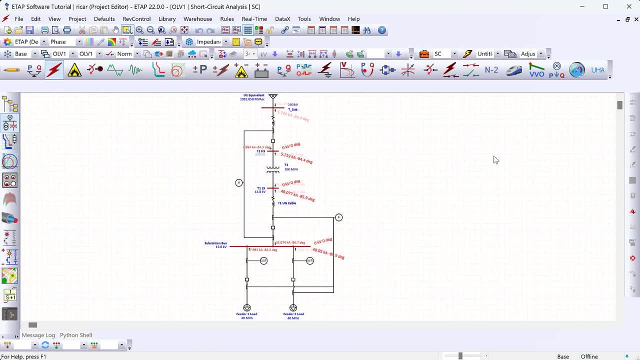 you can have maximum and minimum values. for the most part, you're going to be using maximum values, and what I want to show you over here is this: gives us the fault: current levels for every bus at the substation, in this case, or every bus in your model Now, for example, I'm 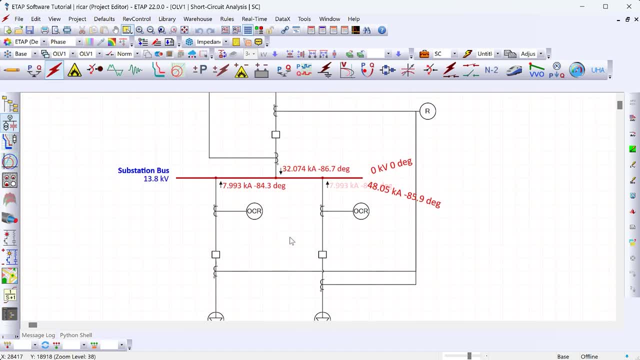 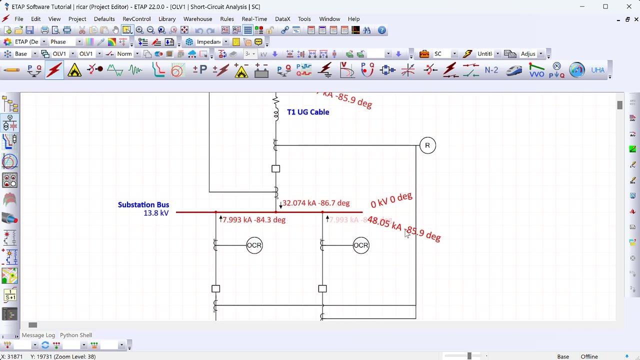 going to zoom in over here to the substation bus and you can see over here that the total fault current for a fault at this bus is 48 000 amps or 48 ka. ETAB typically displays current levels in ka in kiloamps instead of just amps. so this is the total full current 48 ka, and it also 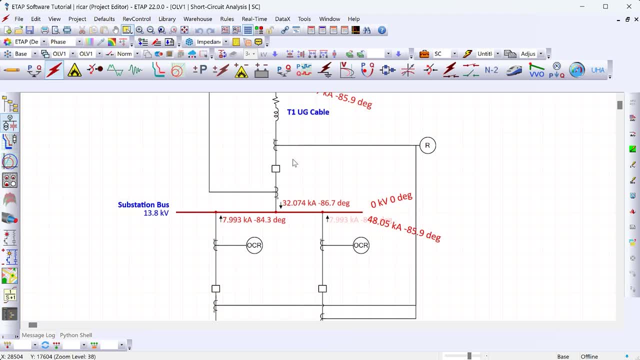 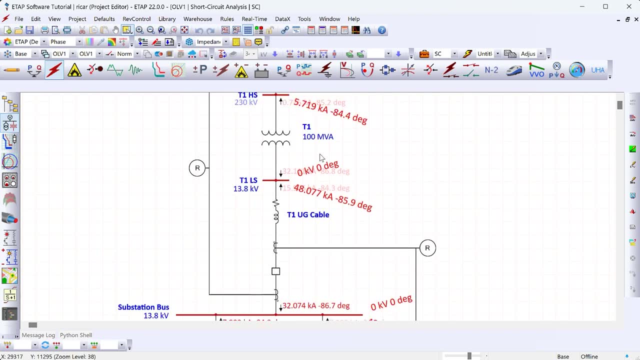 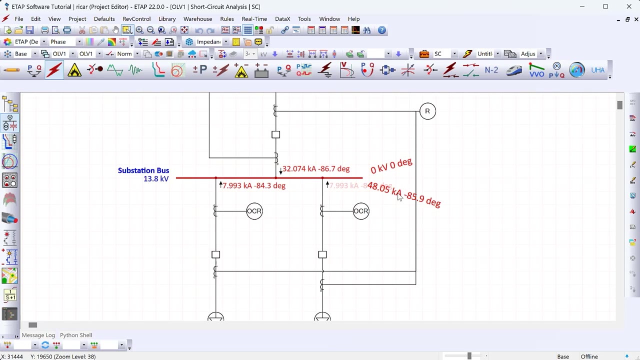 shows us the contribution coming from each side of the system. so we can see that 32 ka is coming from the transformer over here, which of course comes from this utility equivalent, and then we can see the contribution from the induction motors and that, of course, all of that adds up to 48 ka. 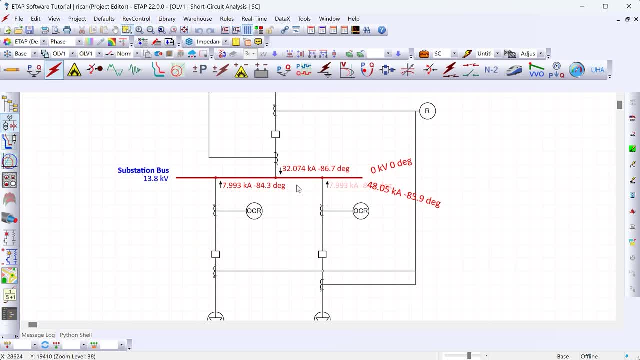 Now, one of the reasons why you might want to run a short circuit study like this is: let's say, for example, that this is a switch gear. this 13.8 kV bus is actually a switch gear. That switch gear is going to have a rating of the amount of fault current that I can withstand during a fault. So for 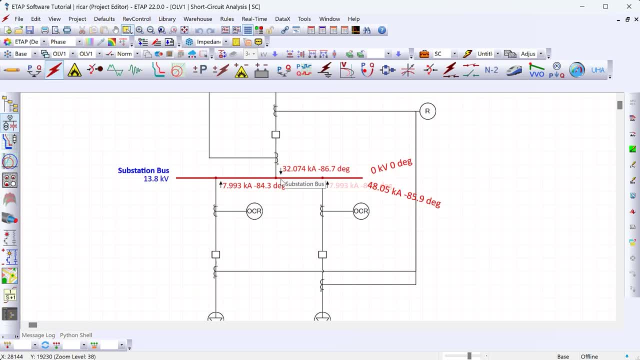 example, there might be a rating for this switch gear of 50 ka and you want to make sure that during the absolute worst case fault in that switch gear, that you're not going to exceed the ratings of the switch gear. That's one of the applications where you might want to run a short circuit study like this. 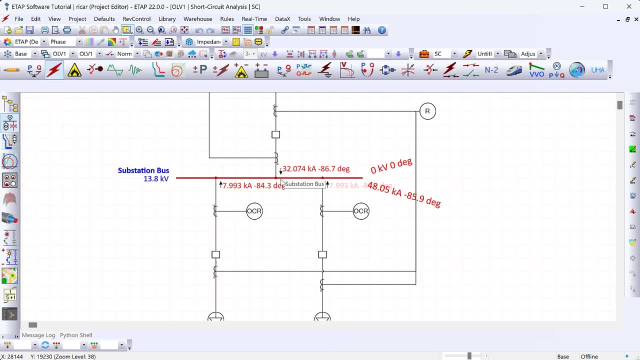 and just as another example. for example had a project in which we had two switch gears tied by a tiebreaker and we found out that if you paralleled the two transformers, the fault current level was too high for any one switch gear to withstand that, so we had to implement an interlocking. 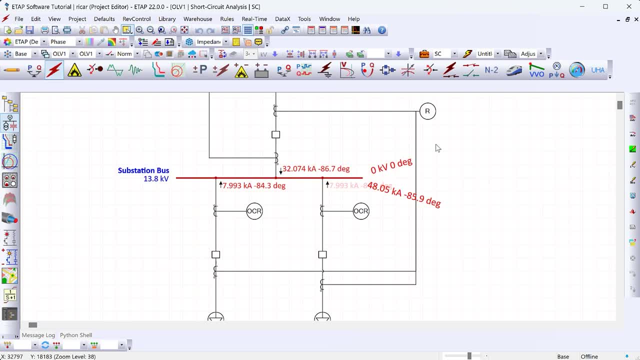 system where the transformers could not be paralleled, such that if there was a fault at the switch gear we wouldЕ over here wouldn't exceed its rating. So that's just a typical scenario where you might want to run a short-circuit study like. 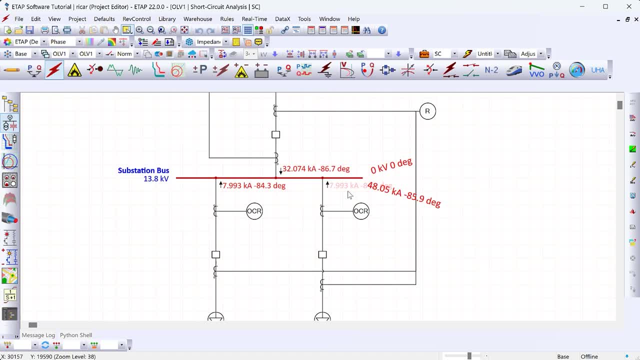 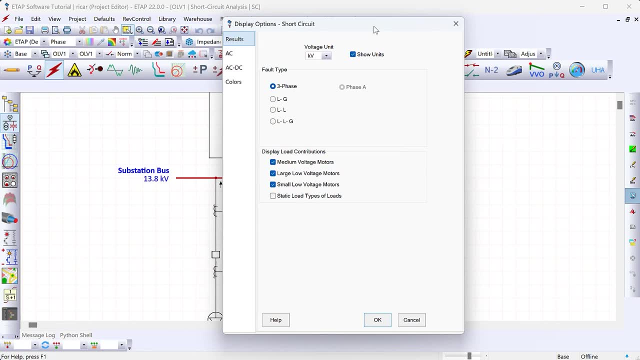 this. Now, the other thing over here is that this information that's being displayed is for a three-phase fault, So you can click on this icon over here and that's going to bring up this window over here, and when you run the short-circuit study, ETAP actually runs all the different types. 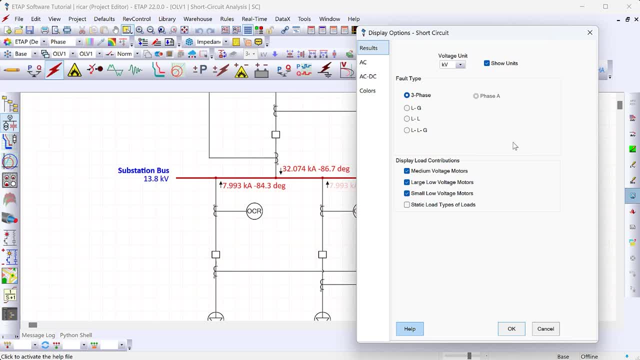 of faults. So it runs three-phase faults- line-to-ground, line-to-line and line-to-line-to-ground- And then you tell it what you want to display in the results. So in this case, I told it run the fault and display the three-phase values. 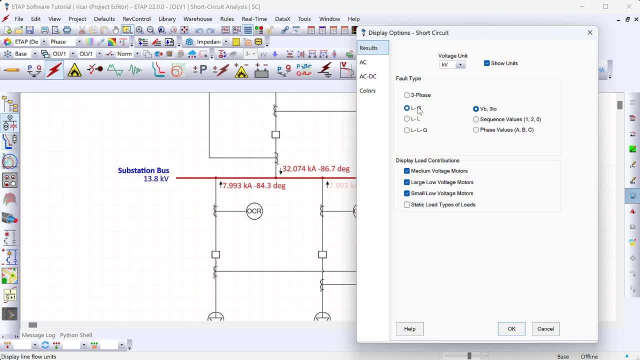 Now I could also switch this to, let's say, for example, line-to-ground, and if you do that, ETAP gives you the option of selecting: okay, which current do you want to display? Do you want to display 3i0, which, of course, is very helpful for protection coordination. 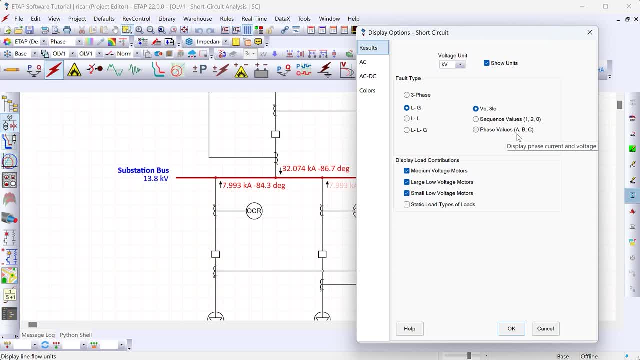 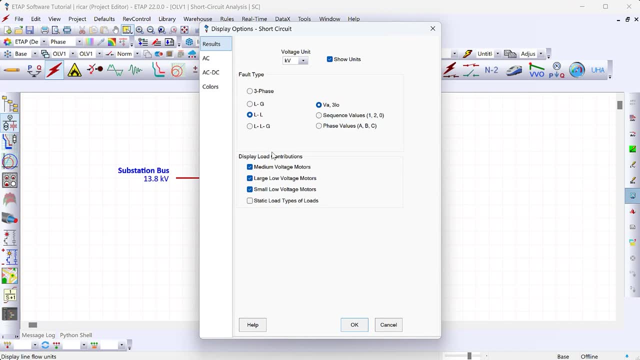 or do you want to display the phase values? In this case, let's say that I want to display 3i0, and then this would be the numbers, And of course, you can also display 3i0.. This would change to line-to-line or line-to-line-to-ground. 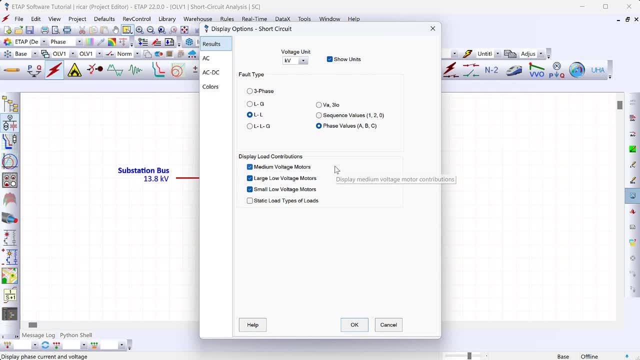 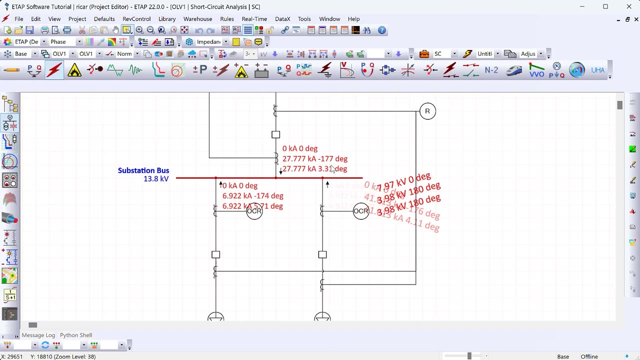 So, for example, for line-to-line, I can select that and I can say: well, I want the phase values, not 3i0.. So let's go ahead and click OK. and now I can see all the individual phase values. For example, the contribution from the transformer in this case would be 0 kiloamps for A phase. 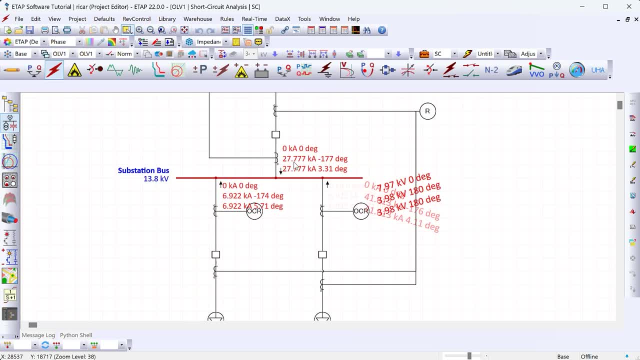 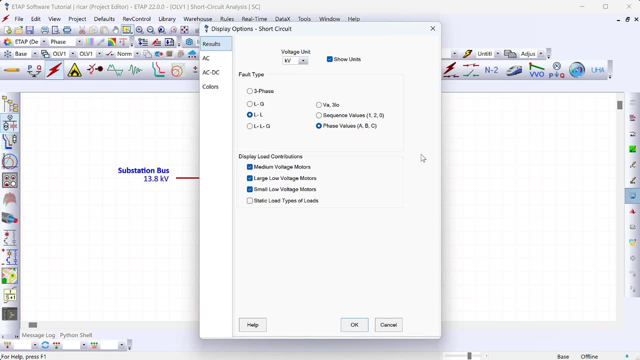 and 27.8 ka for both B and C phases. Of course, in this case we ran a B to C line-to-line fault, So it's just different types of results that you can display Again if you want to see the maximum fault current level. that's typically a three-phase. 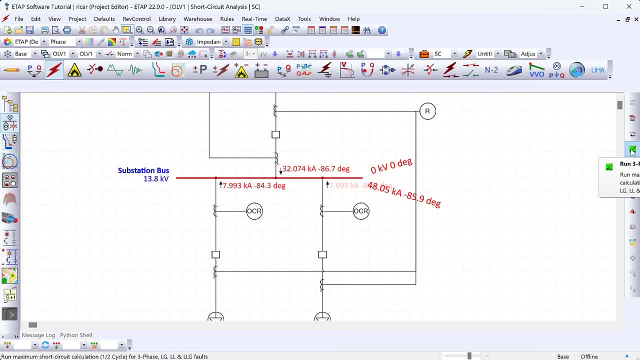 fault current and you would select over here the max short circuit such that all the transients are taken into account. All right, so now let's move to protection coordination, and that is under this module over here which is called start protection coordination. Let's go ahead and click on that and again we have our model over here where we have: 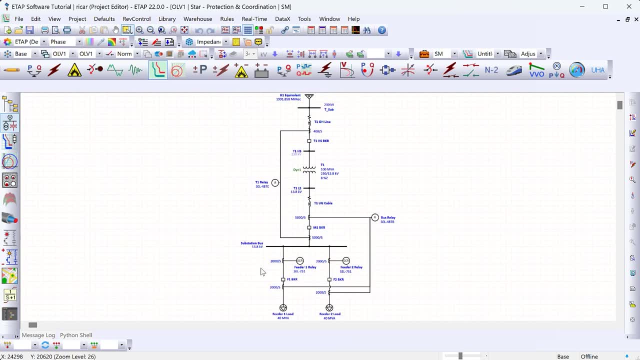 a utility equivalent. We have a transformer substation bus, two feeders. What I want to do for this is: I'm going to go ahead and click on that and again we have our model over here, where we have a utility equivalent. We have a transformer substation bus, two feeders. 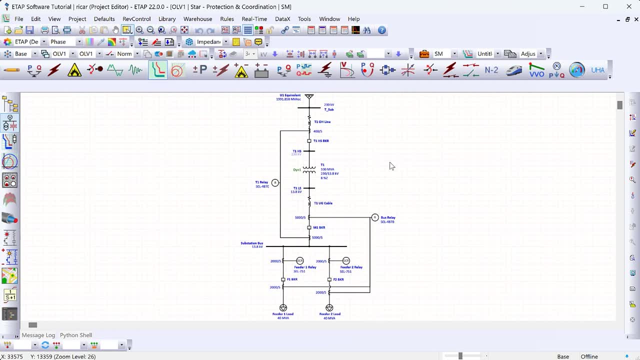 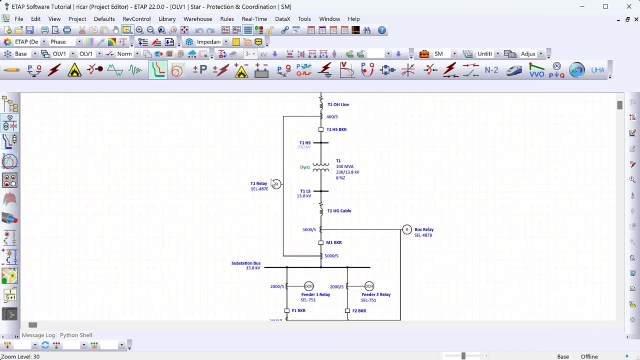 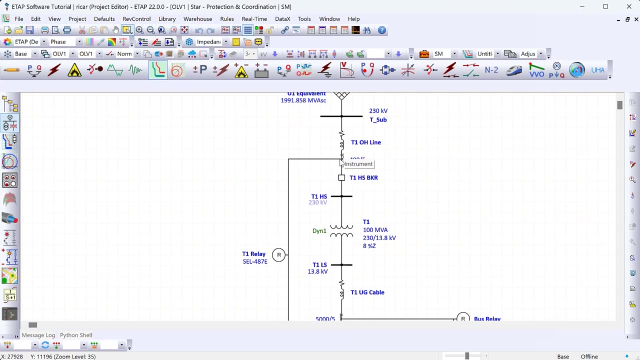 What I want to do for this example is show you how to do a protection coordination where we have an overcurrent element on this relay over here, which is an SCL487E that is implemented on the high side of the transformer. So it's going to be reading the current off of this CT over here and it's going to 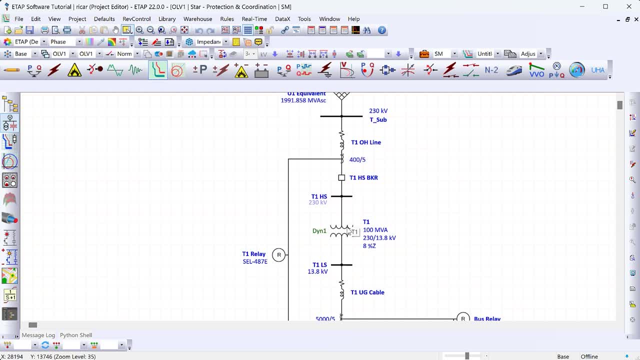 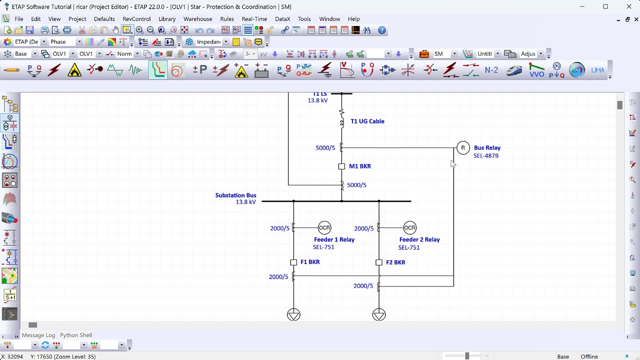 implement an overcurrent that's both going to protect the transformer and the substation bus, and then we're going to coordinate that with this feeder, one relay over here, and we're going to display the curves and see how we can perform the coordination. Now I'm going to skip this bus for this example. we're going to assume that that's just doing. 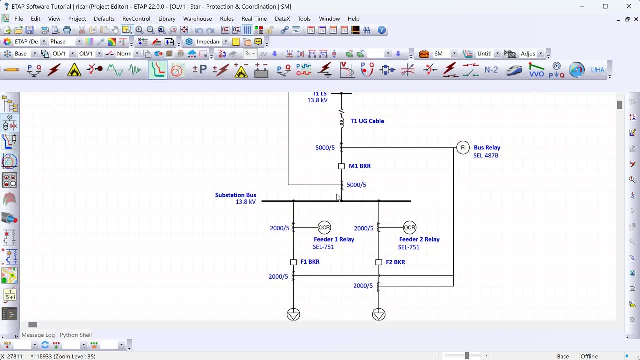 bus differential protection for this substation bus and it doesn't have overcurrent elements. In this case, the 51 or inverse time overcurrent element that we're going to be implementing here on the high side of the transformer would also provide backup for faults in the substation. 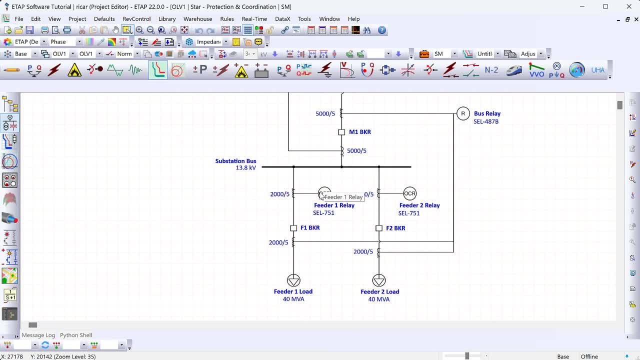 bus and then we're going to coordinate that with the inverse time overcurrent element in the feeder relay over here. So let's go ahead and do that again. I have an SCL487E relay for the transformer and an SCL751 relay for the feeder relay. 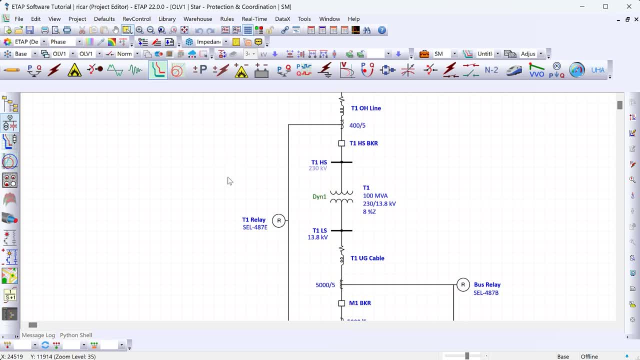 Now again, I've gone ahead and modeled this and we showed that in the previous video. but this relay over here of course has two CTs, one on the high side and one on the low side, and again the overcurrent is going to be reading off of the high side CT. 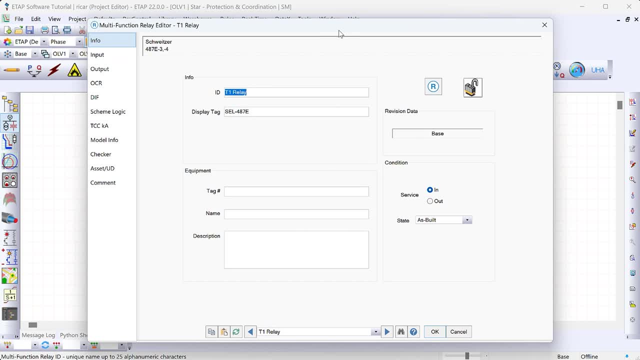 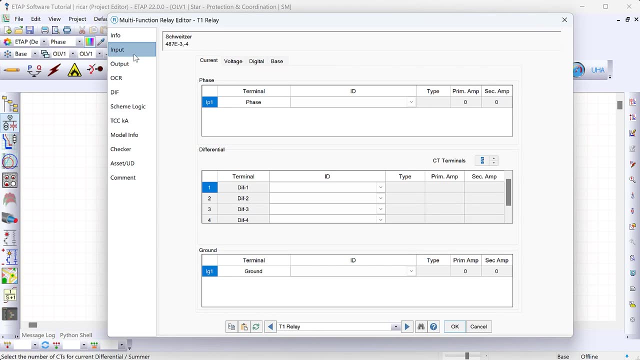 So let's go ahead and click on this SCL487E relay and we get this window over here. The first thing that I want to do is to make sure that the input tab over here is set up properly. So this is where ETAB gets the information as to what CT to use. 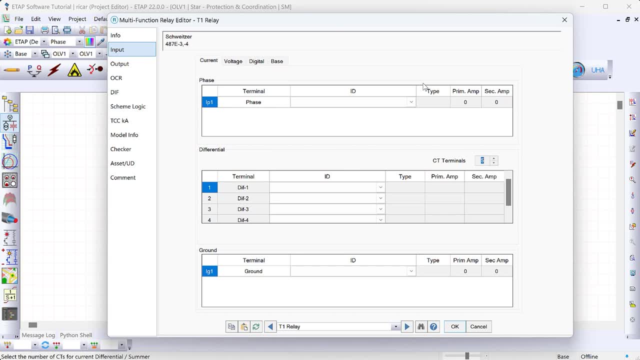 for what element In this case? let's say that we're just going to be implementing a phase over current element And that's going to be reading the CT on the high side of the transformer. Now notice over here that it gives me two options, And that is, of course, because 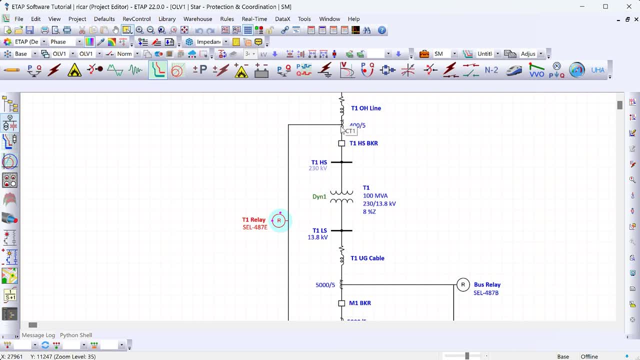 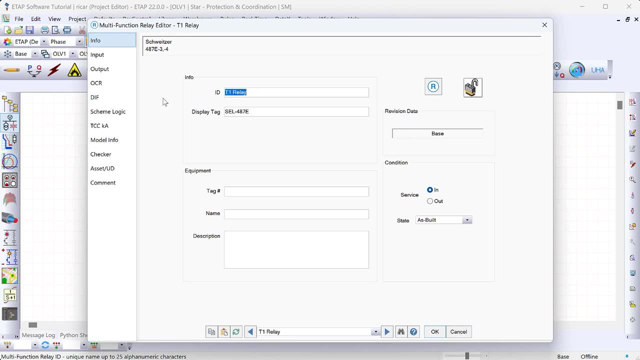 we have two CTs. This one at the top is called CT1. And this one at the bottom is called CT5. So when I go over here to the input tab and I click on this drop down, it gives me those two. 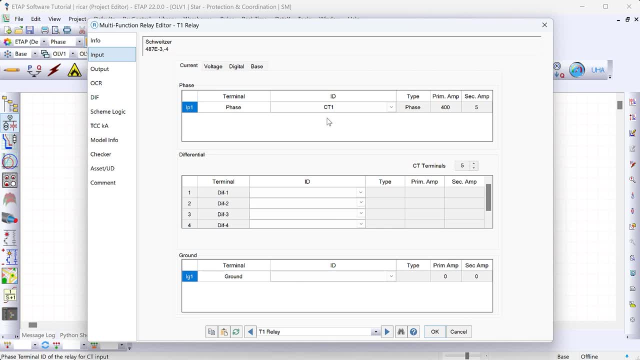 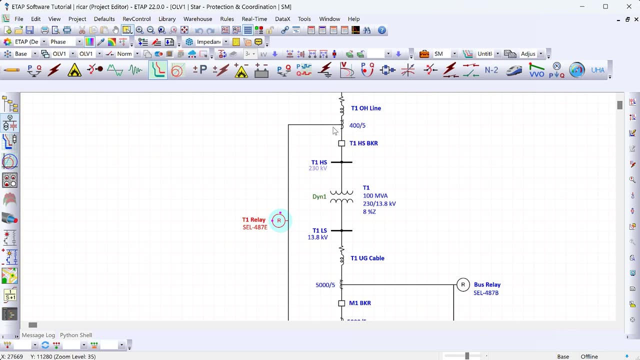 options. In this case, again, we want our over current element to be on high side CT. So I'm going to select CT1. And we can verify over here that that's 400 to five, which of course is the ratio for this high side CT. Now I want to do the same thing for the feeder relays. So if I double, 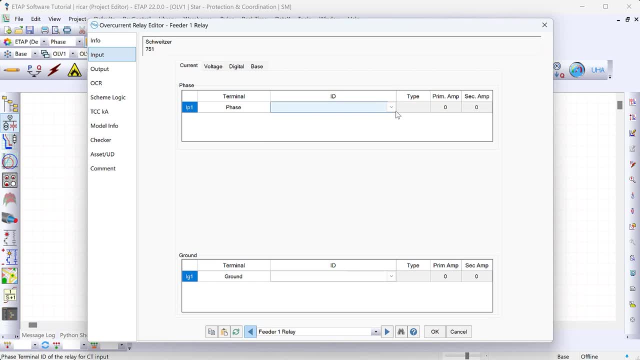 click on this feeder, one relay, and I go to input and I select this drop down. here, of course, we only get one option because there's only one CT that is wired into the relay. So we can just click on that And again it displays: now here, 2005.. And if we go back to our model, 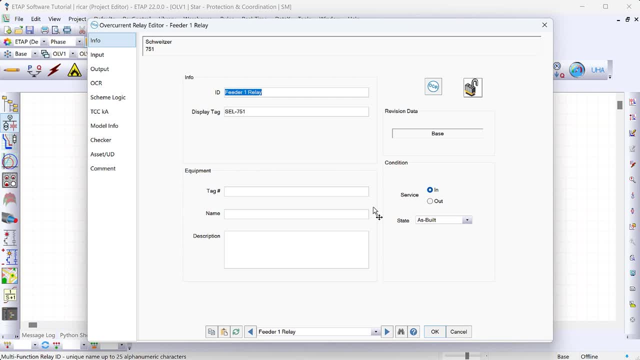 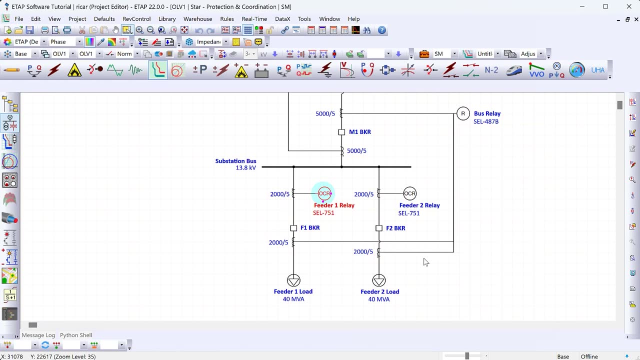 we can see that, of course, that matches this number over here. So we've set up the CTs for each one of the relays. The next thing that I want to do is to enable the over current elements on each one of the relays. So let's do the 47E first. let's double click on this. 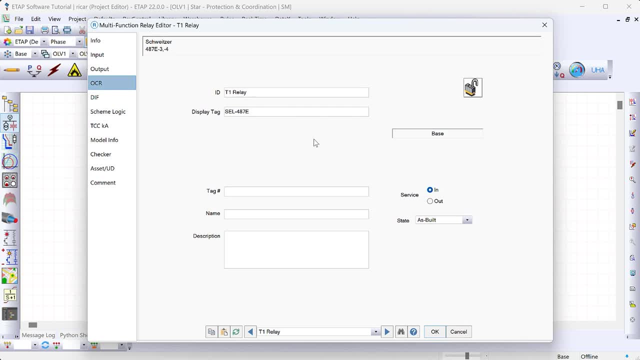 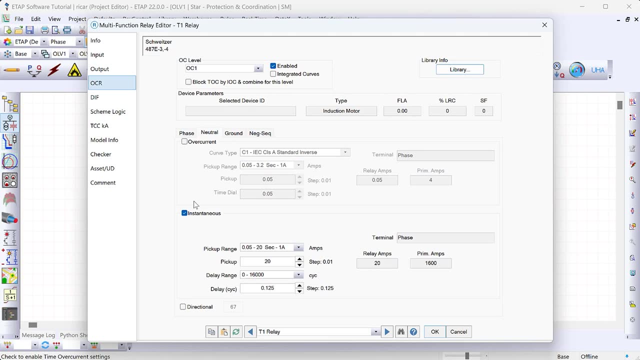 And now we can go over here to OCR And by default there's a bunch of things here enabled. I'm going to disable all of this Again. for this example, we're just going to do a phase over current element And for this relay specifically, we're going to have both a 51P. 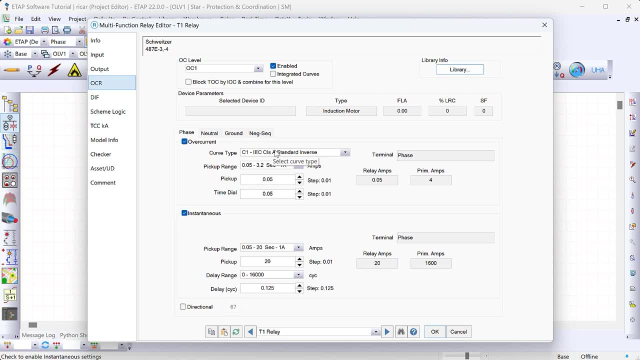 element. so an inverse time over current element and an instantaneous over current element. both are going to be phase elements, So I'm going to disable negative sequence, ground neutral, just leave the phase on And I'm going to have both inverse time. 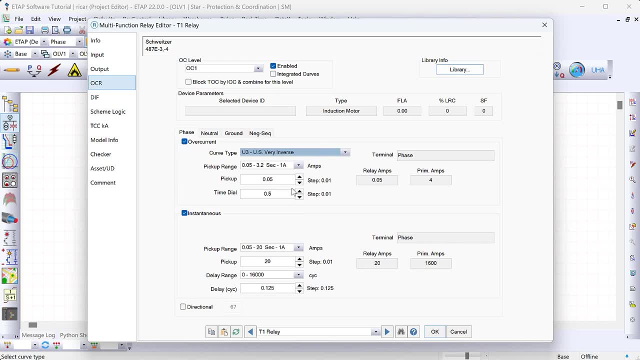 and instantaneous. Now for this example. I'm going to use U3 curves for the 51 elements. I'm going to assume that this is a five amp CT and we have to select the pickup and the time dial. I'm going to leave those at default for now, And let's go ahead and do the same thing. 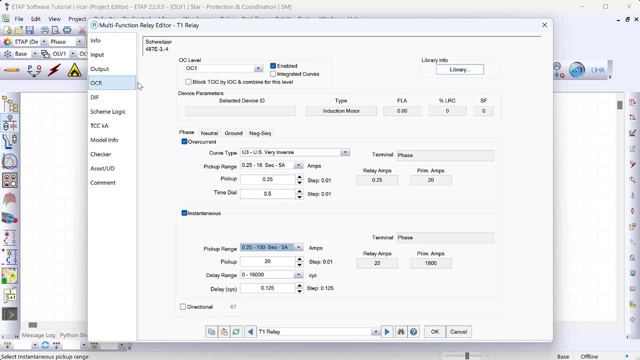 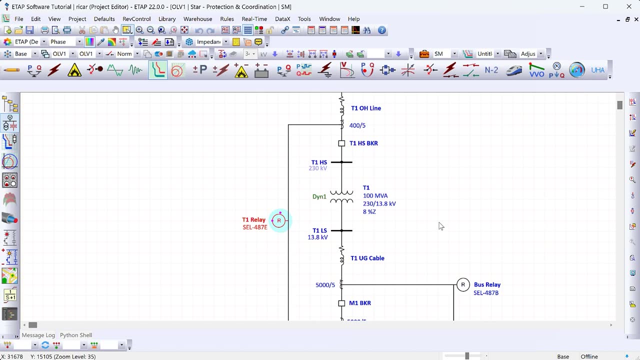 for the instantaneous. that's going to be a five amp relay, So now I enable both 51 and 50, both phase elements. I'm going to click OK, let's go to the feeder relay now And let's do the same. 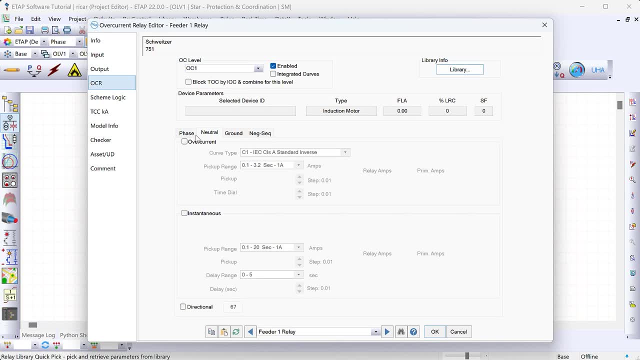 again, I'm going to disable everything that is not a phase element, And in this case it looks like everything by default is disabled for this relay, And let's go ahead and change this again to U3, five amps And for the feeder. I'm not going to have an instantaneous element, So I'm 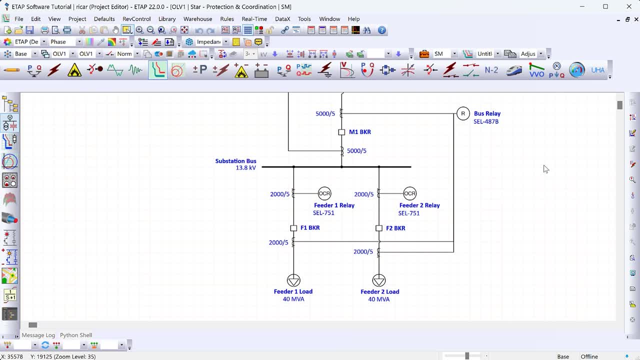 going to uncheck the instantaneous box over here, Alright. so what we've done here is we've told ETAP which CT to use for each relay, we've told it what kind of element- protection element- we want to use for each relay, And we're going to disable everything that is not a phase element. 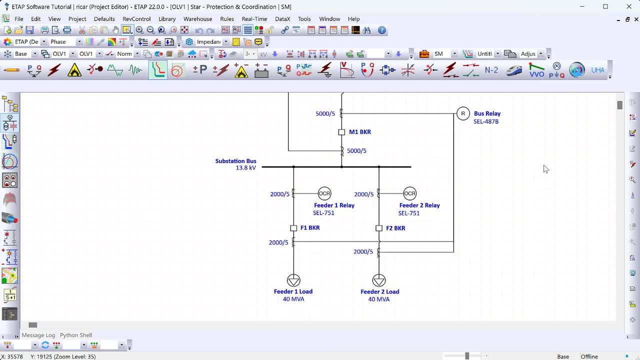 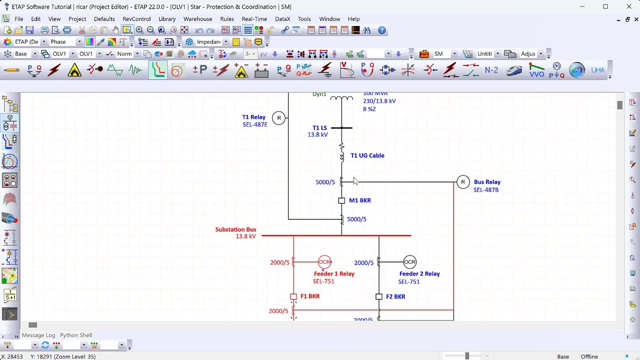 We want. So now we can put this in a TCC, a time current characteristic plot, and do the coordination. So what I want to do here is you can select everything that you want to be included in the plot. So in this case it's going to be the feeder all the way down to the load this bus. 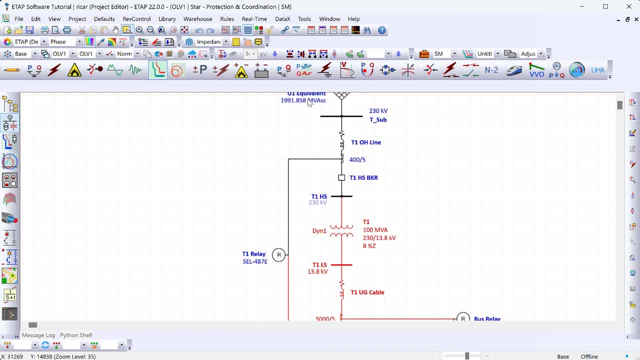 and then everything over here, Let's say up to the utility equivalent, And let's also include this relay And our feeder. one really was also included. So I've selected everything that I want to be included in my TCC plot. So once you do that, 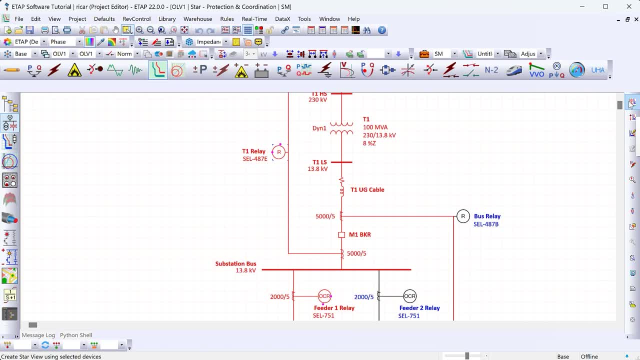 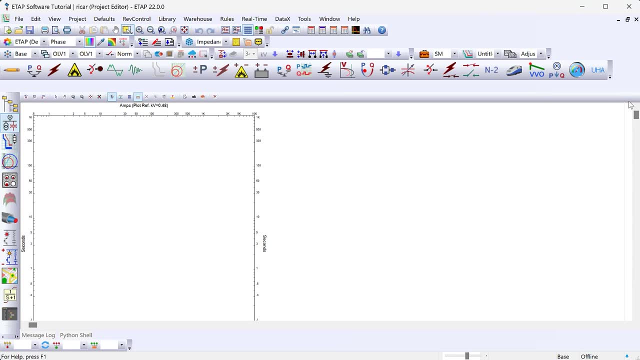 you can click on this button over here, which is to create a star view. A star view is basically the TCC plot in ETAP, So let's go ahead and click on that. And now ETAP is going to create this plot. 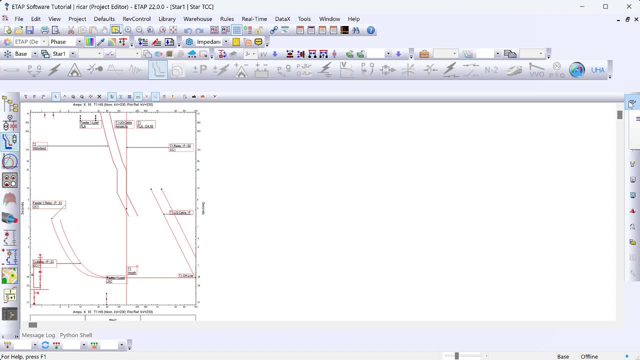 and it's going to put everything that we selected into this plot, including all the equipment. So you can see over here that we have the damage curve, for example, for the transformer, for the cables, And then we have our elements over here that we enabled. 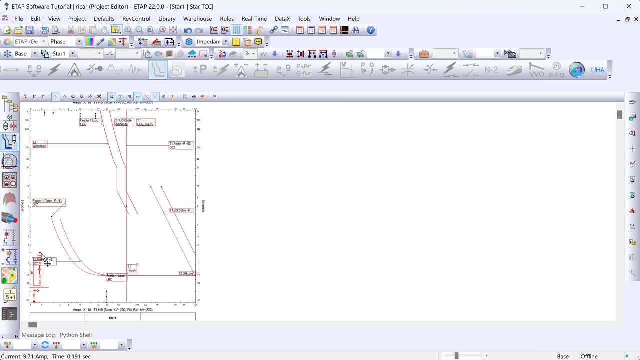 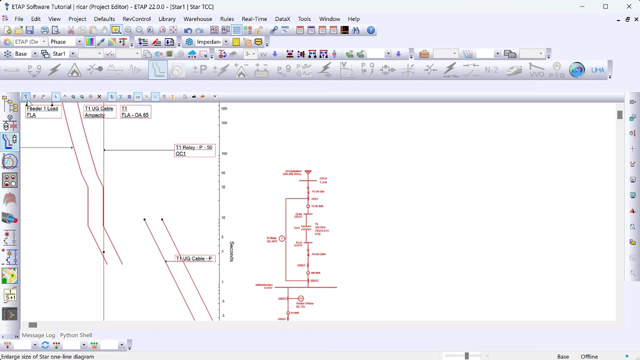 So the first thing that I want to do over here is just select this one line over here- And let me actually make that a little bit bigger, just so it is easier to see- And in here you can select that and then click on this button over here And that's going to make this one line view a little bit. 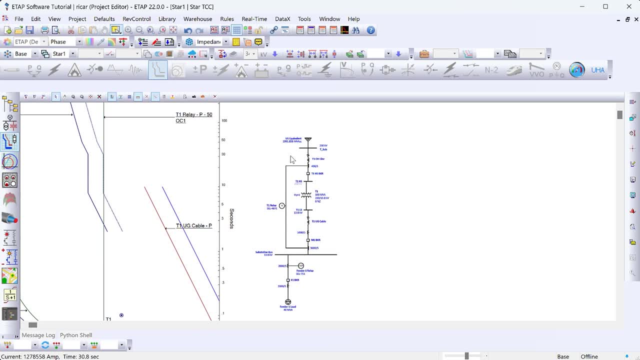 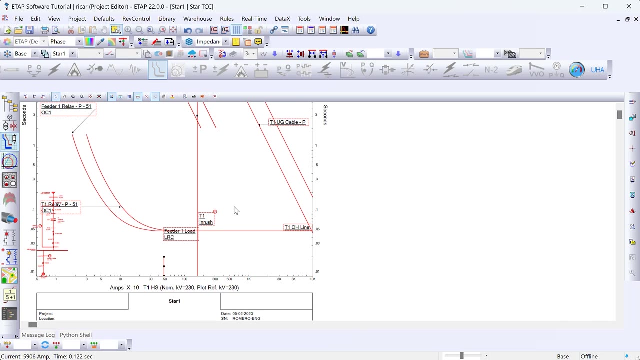 bigger, just so that we can see where everything is at. So again, we selected everything down to the feeder Over here and we're displaying here basically a one line of the curves that we're going to be displaying in our TCC plot. So now I'm going to move that over here And typically I like to put 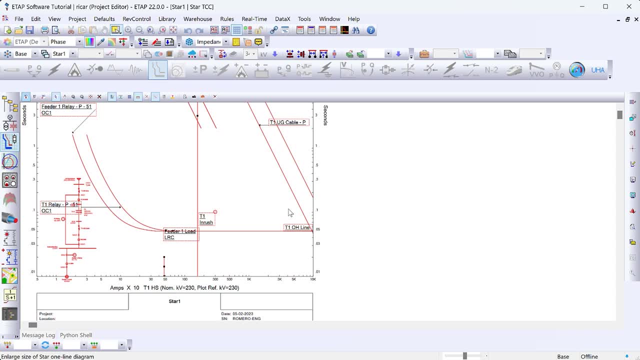 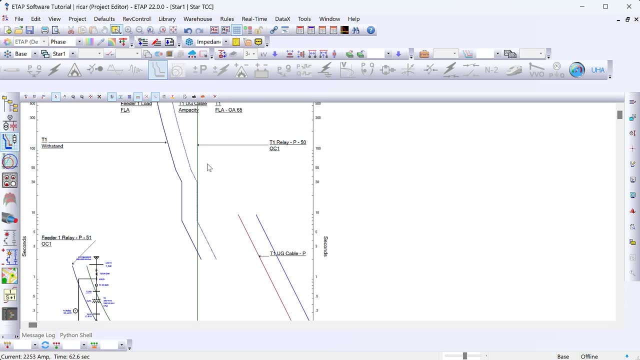 this here on the bottom left just to kind of reference what's shown here on the plot. All right, Now, this is a little bit crowded over here. The reason for that is that we haven't actually set our overcurrent elements, So you can see that the curves are all the way down over here. 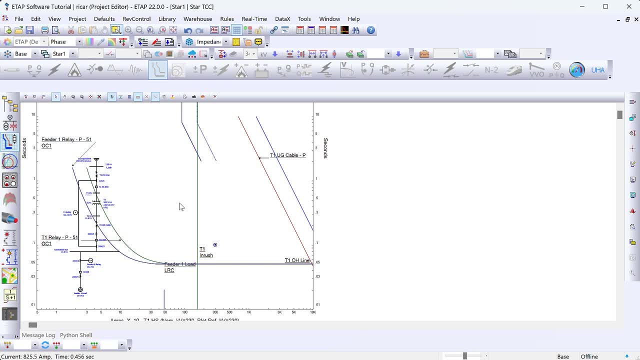 That's just because we haven't actually put values in our settings, So let's go ahead and do that. The first thing that I want to do is select the pickup for our high side time over current element on the SEL487E. Now to do that, we're. 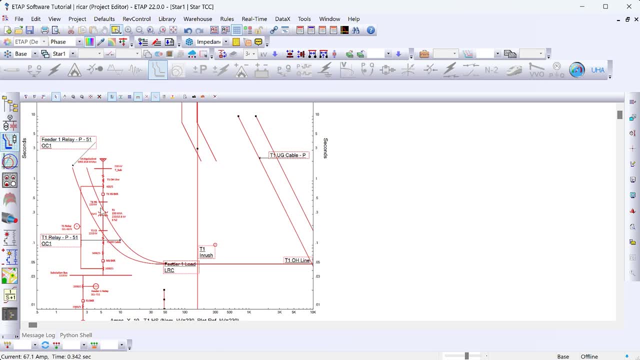 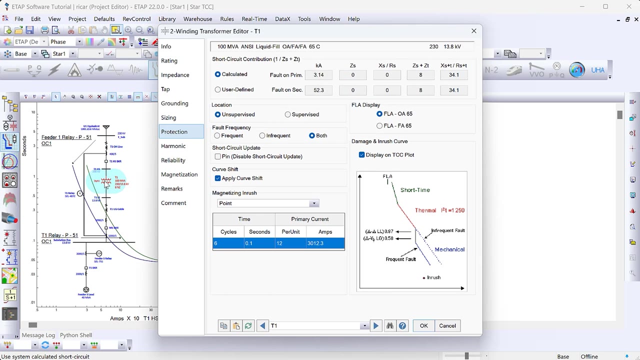 going to do a couple of things. One is that- and let me actually make this just one click bigger Again- we know that we have a 400 to 5 CT on the high side of the transformer and we have a 100 MVA transformer. Now, the maximum rating for this transformer per standard. 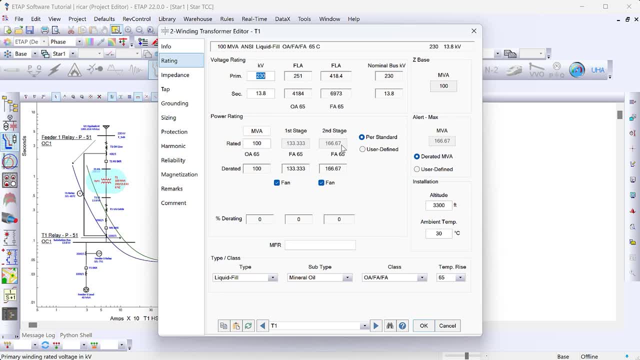 is 166.67 MVA. So we want to select the pickup of our inverse time over current element on the high side of the transformer to be some margin above that value. In this case I want that to be 25% above that value And ETAB actually displays the full load amps for that MVA over. 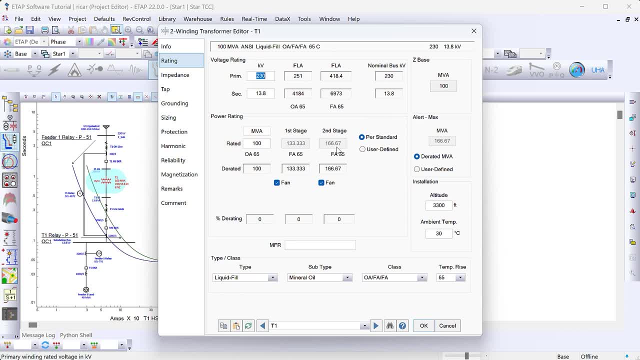 here. So we can see basically that at 230 kV, 166 MVA equals 418 amps. So what I want to do for my SEL487E is I want to set the pickup of the time over current element to be 25% higher than that. 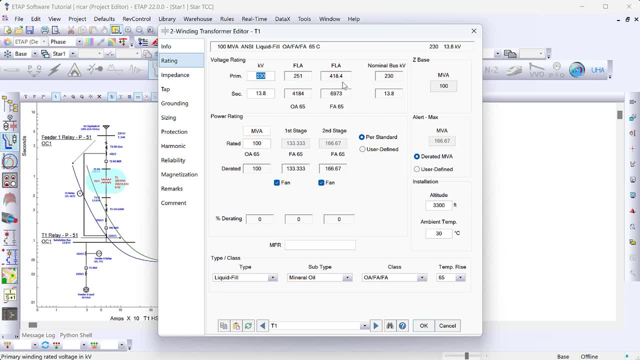 So this number 418 times 1.25.. And then, of course, we need to convert that to secondary amps based on the CT ratio that we have. So let's go ahead and do that Again. that number is 418.4.. And let 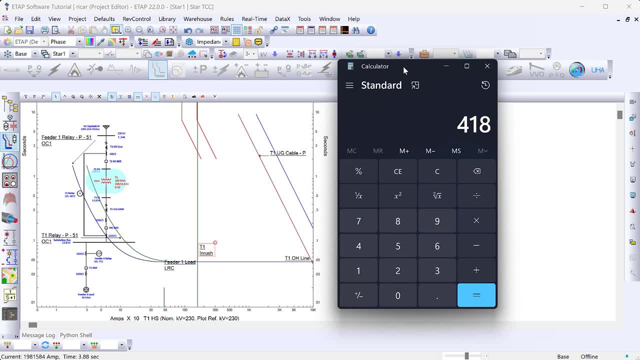 me pull up my calculator over here. So again we have 418.4.. We're going to multiply that times 1.25 to give us some margin above that value, And then I'm going to divide that by the CT ratio for that over current element. 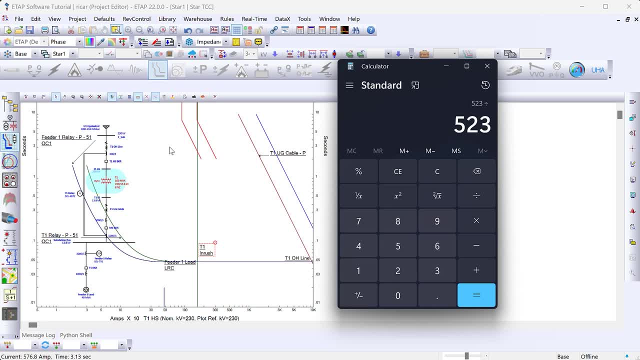 which in our case is 400, to 5,, which is 80. So I'm going to divide this number by 80. And that gives me 6.54.. I'm going to round this to two decimal places. So our pickup is going to be: 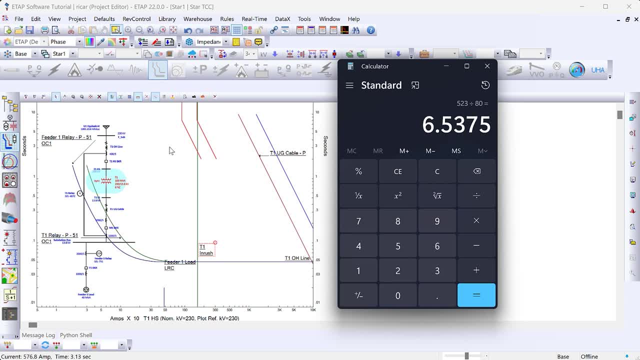 6.54.. Again, that equates to 25% above the maximum rating of the transformer that we have, And that's of course because we want to make sure that we don't trip on load. So 6.54,. 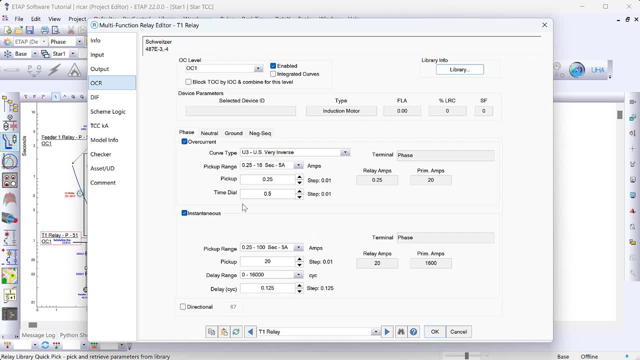 now we can go into my relay over here And my pickup is going to be 6.54.. I'm going to go ahead and click OK. And now you can see how that curve moved from here all the way to here. Now the other. 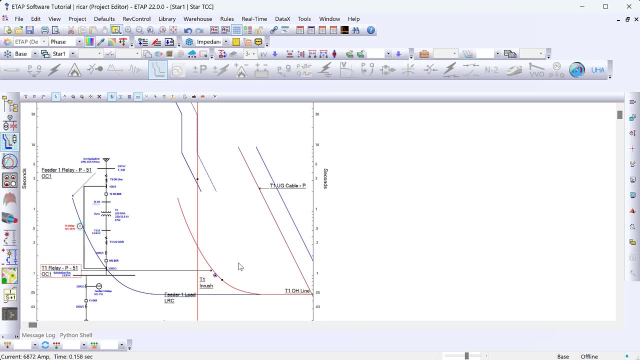 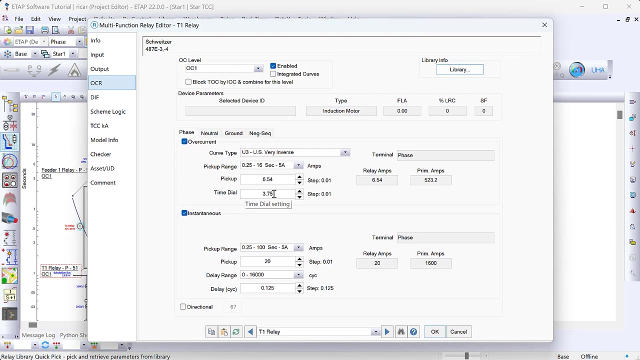 thing that of course we want to do is to set the time dial of this over current element. you can actually drag the curve over here to any point on the curve And that's automatically going to update the time dial that's over here. So in this case I move that curve all the way up and that gives me. 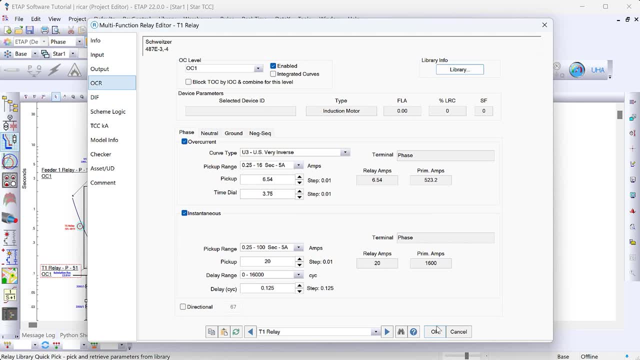 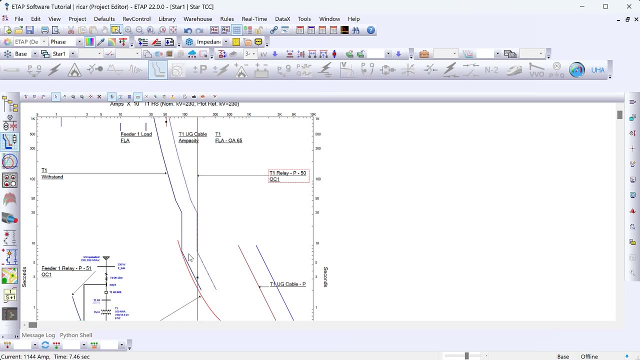 a time dial of 3.75.. And let me actually go back to the plot And the reason why I want that time dial is because we have the damage curve of the transformer down here and I want to be just below that damage curve. So again, we selected the pickup based on the rating of the transformer to make. 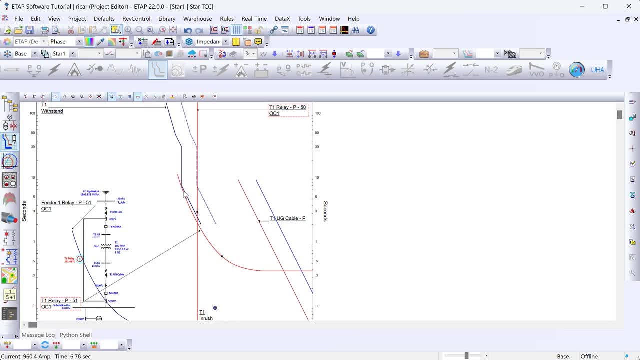 sure we don't trip on load Now the time dial. I'm going to select it based on the fact that I want to coordinate with the damage of the transformer, which is this one over here. so that gives me a pickup of 6.54. let me actually 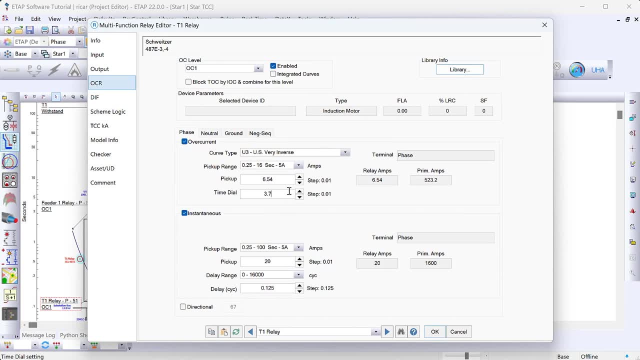 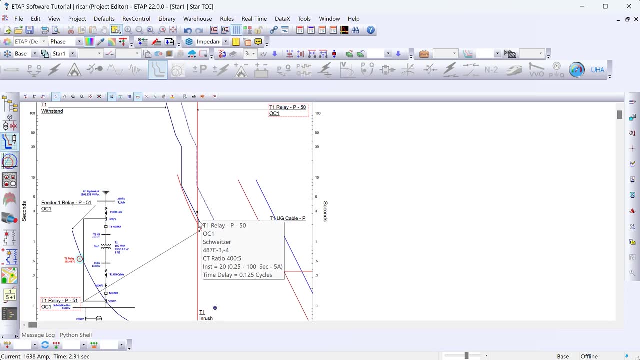 move this down just a little bit to have a little bit more room in there. so I'm going to select 3.7 and, as you can see, that puts the curve for that 51 element on the high side of the transformer just below the damage curve for the transformer. to make sure we also protect the transformer. 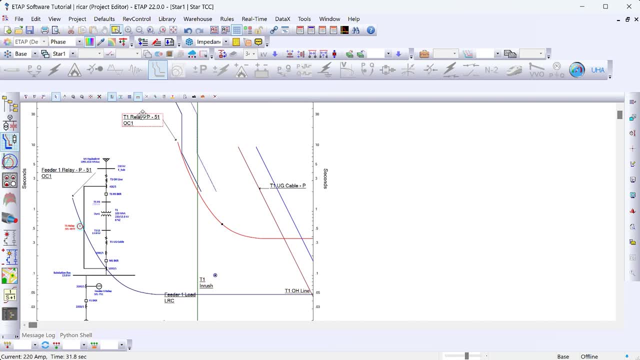 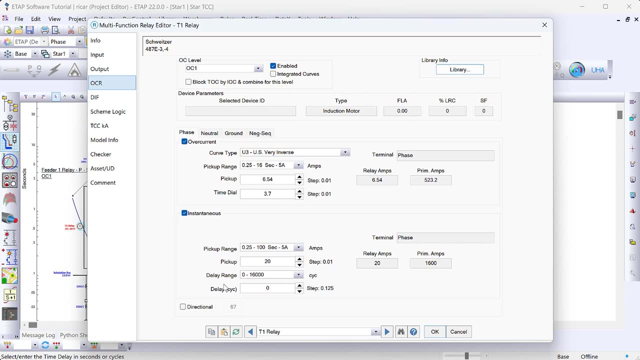 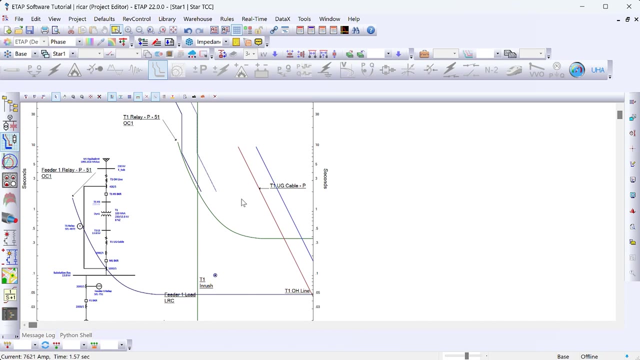 Now I also said that we want an instantaneous over current element on this relay over here, which right now set to the default of 20 amps, and I actually want this to be instantaneous. so zero cycles for the delay. and to select that we have to do two things. one is we need to run a fault on the. 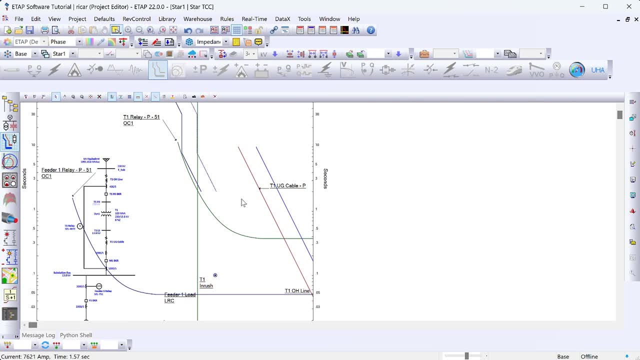 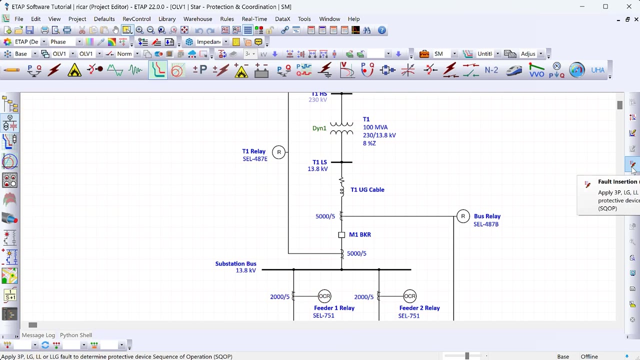 low side of the transformer and make sure that we select the pickup such that that's above that value. and that is just to make sure that we don't trip instantaneously for a fault on the low side of the transformer. So if I go back over here to my model, what I can do from this star view is put this fault in here. 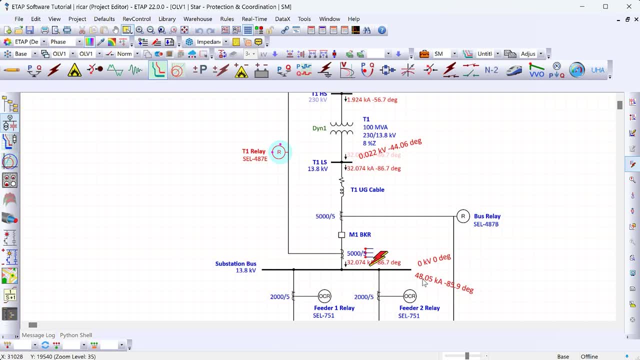 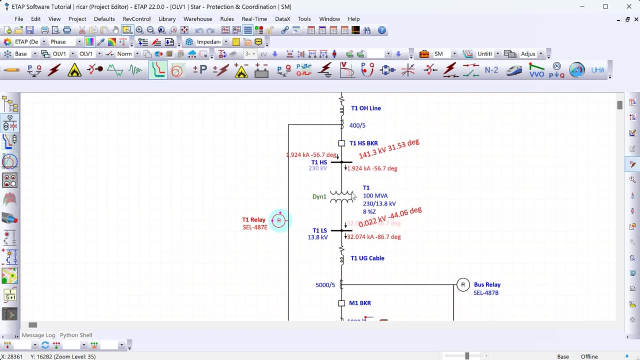 and let me actually get rid of this. and again, this is the number that we saw before: 48 ka total, 32 ka contribution from the transformer. now that's on the low side of the transformer. and again, remember that our relay is reading current off of this ct. 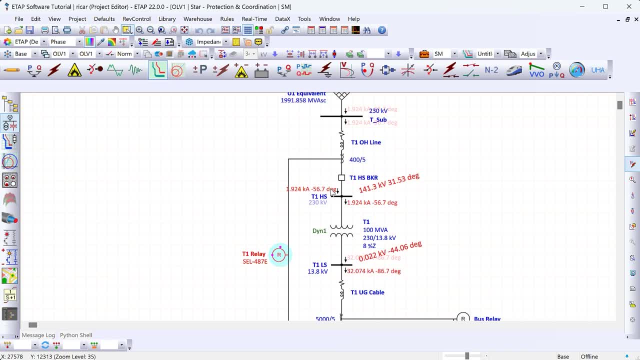 so the contribution on the high side, basically at 230 kv in this case, is going to be the low side of the transformer and again, remember that our relay is reading current off of this ct. so the contribution on the high side, basically at 230 kv in this case. 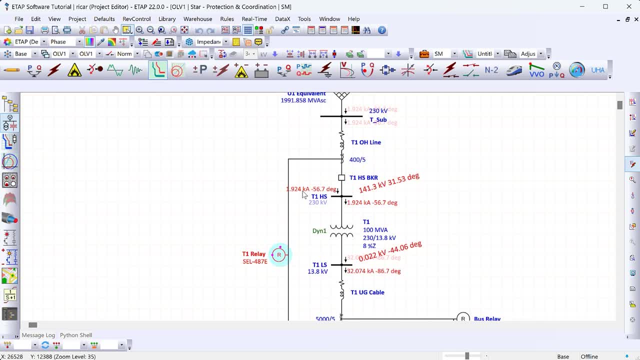 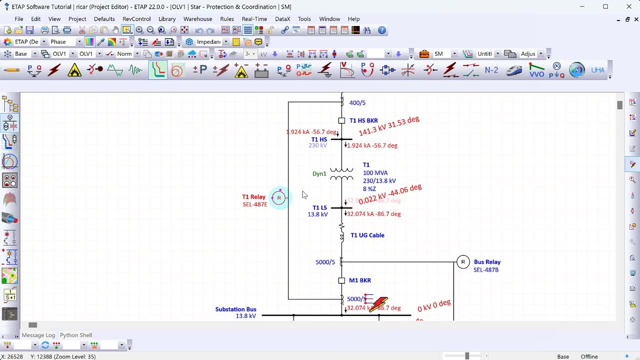 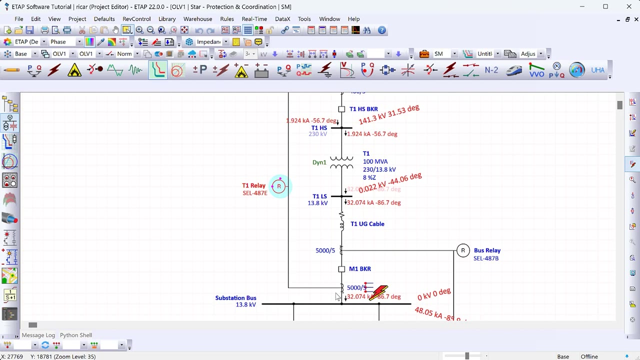 is 1924. so we want to make sure that our setting for the instantaneous element is above that value with some margin, such that we don't trip for a fault here on the low side of the bus instantaneously, because that of course would create miscoordinations. 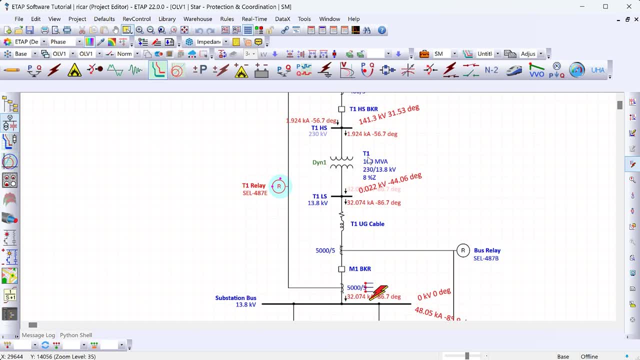 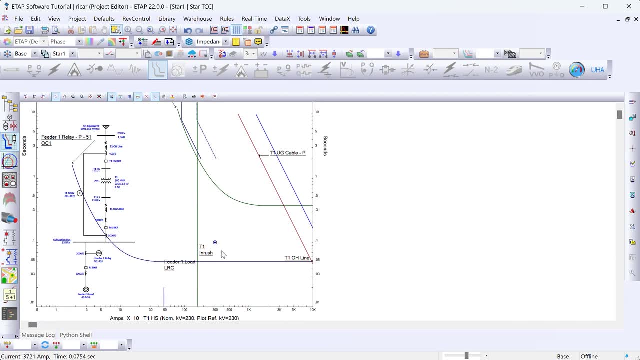 with anything down here on the substation bus. now, the other thing that we want to watch out for- and that's better shown on the tcc- is the fact that we have this inrush point for the transformer. what that is is when you first energize the transformer, you're. 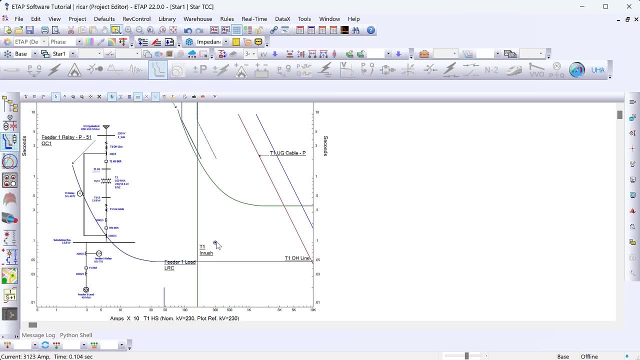 going to see a spike in current just because that's magnetized in the transformer, and so of course we want to make sure that we don't trip for that, because otherwise that would mean that every time we enter the transformer the instantaneous element is going to trip back out, and of course 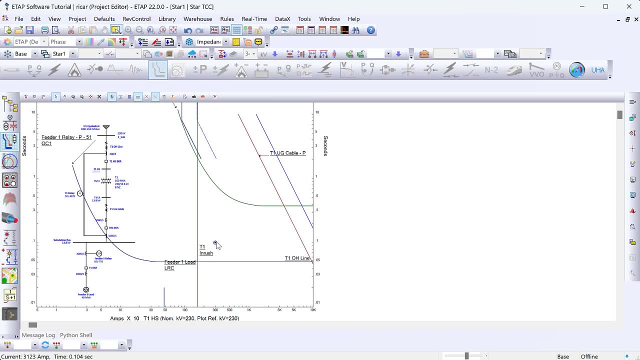 that's something that we don't want. so two things for your instantaneous over current element. one is, again: you want to make sure that you don't trip for a low side fault, but also you want to make sure that you don't trip for inrush. so what i can do here is i'm going to 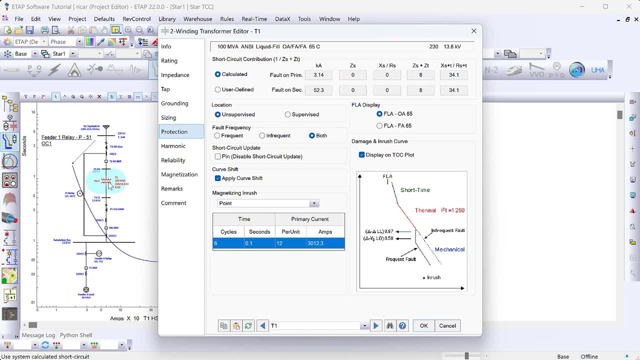 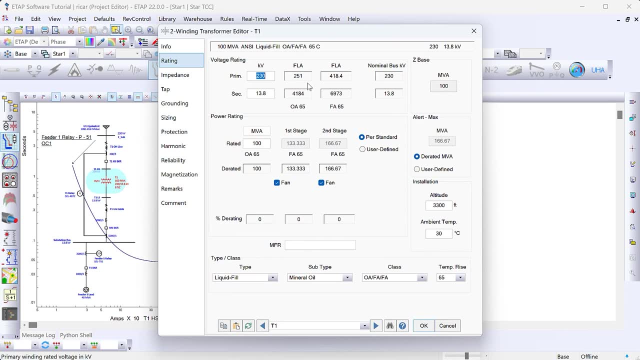 do for that is: i can double click on this transformer, i can go to the rating and i can see that the oa rating, the self-controlled rating, for this transformer is 100 nva. that in current at 230 kv is 251 amps, and a typical rule of thumb for inrush is that the worst case inrush is going to. 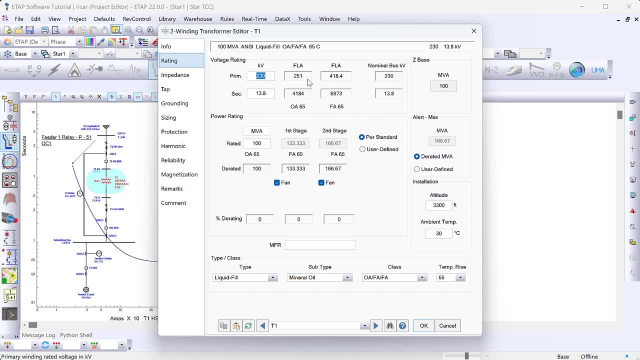 be 12 times the oa rating of the transformer. so basically, if we take that number, multiply that times 12, that's going to be our worstר case and rush, and then we can add some margin on top of that. so let's go ahead and do that i can. 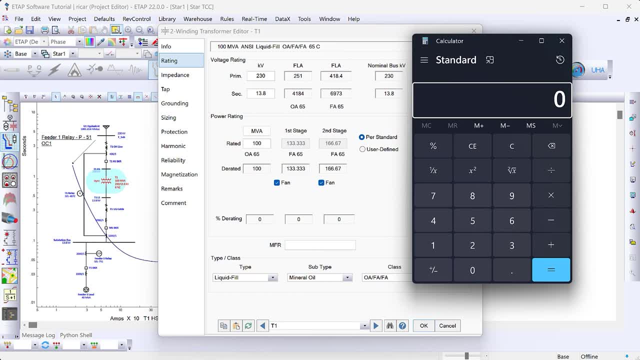 say: well, i'm going to take 251, which is our oa rating current, multiply that times 12 to get my worst case and rush. and then i'm going to add some margin on top of that. i'm going to do 20 above that, and then, of course, we need to convert that back to secondary amps for the relay. so if 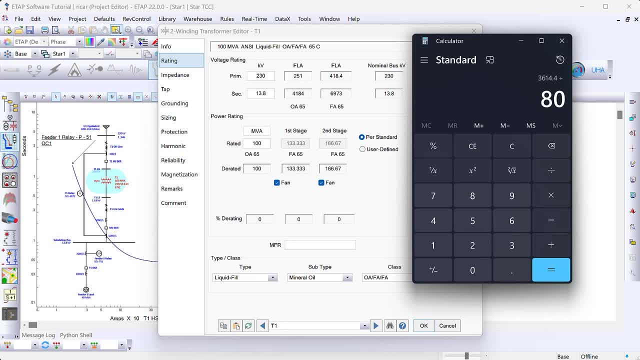 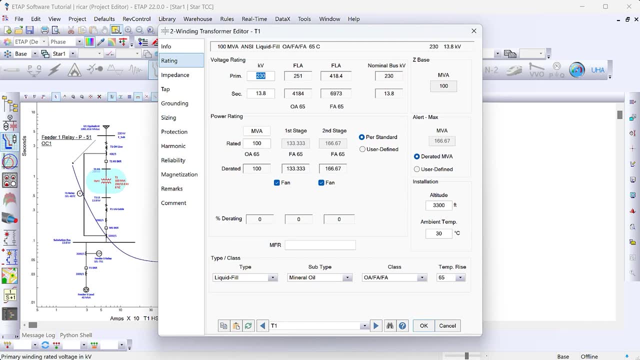 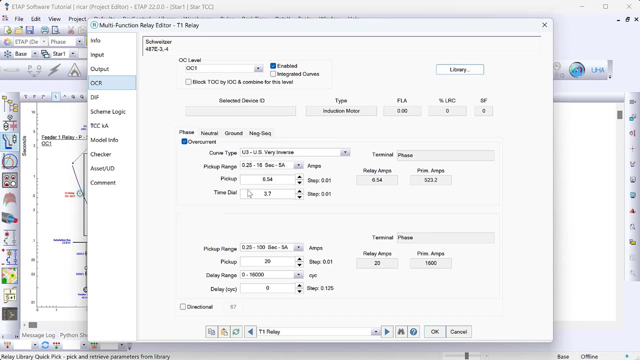 we have a 400 to 5 ct. we're going to divide that by 80 and that gives us 45.18 amps. so my instantaneous element then is going to be 45.18, so we can go back to the 47e relay. so let's double. 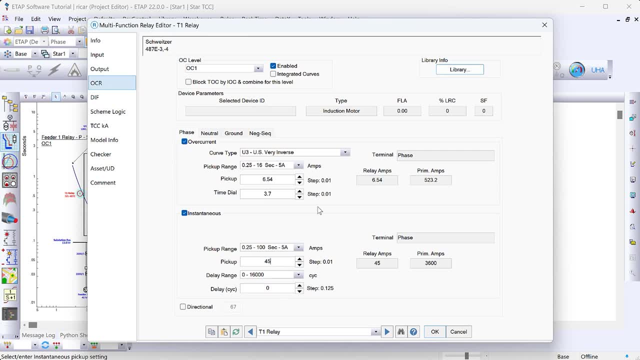 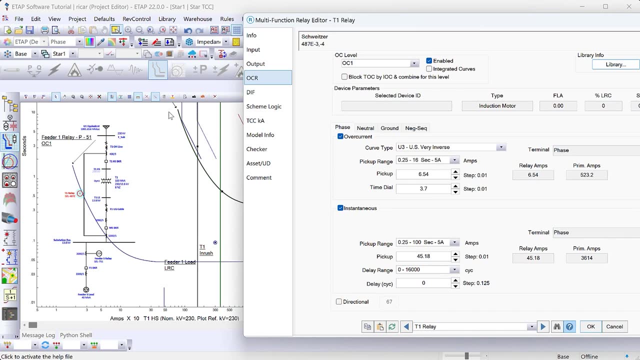 click on that and i'm going to change this number to 45.18. now the other thing that i want to do in this step is notice over here how we have a different curve for the 51 element, and the other thing that i want to do in this step is notice over here how we have a different curve. 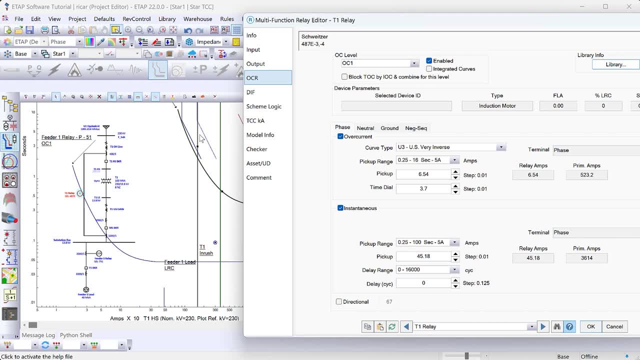 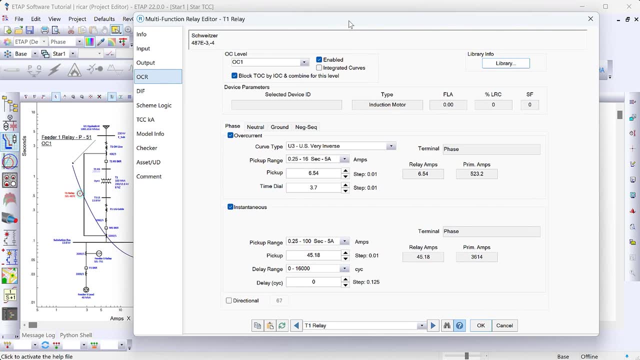 the inverse time over current and the instantaneous over here i want to combine those two. so i'm going to click this box over here which says block toc by ioc and combine for this level. what that does is it's just going to combine the two curves into one. it just makes it easier to read, so let's go. 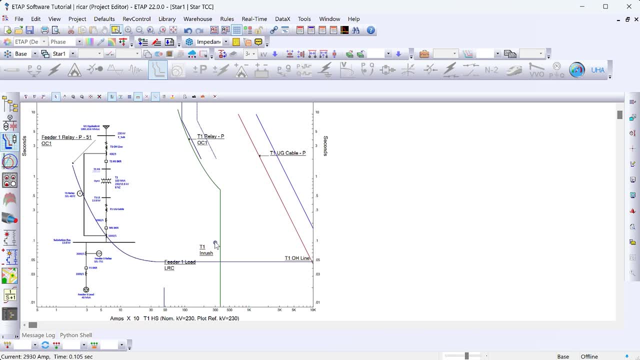 ahead and click ok, and now you can see that we have just one curve that is above in rush. and then we also calculated that that was above the worst case fault for a low side transformer fault. so now we're done with our 50 1p and 50 elements on the transformer. the next thing that we need to do is to select the settings. 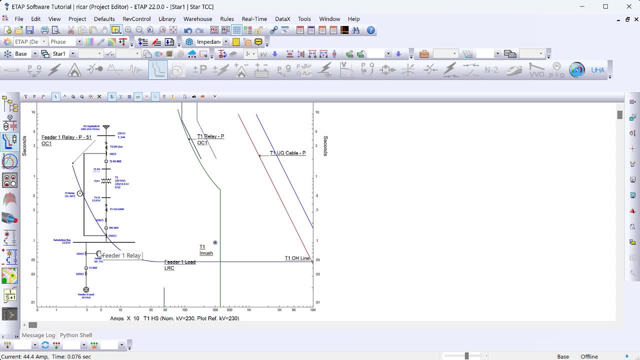 for this feeder relay and then do the coordination. so in this case we have a 40 mba load, and let me actually make this a little bit bigger. so our load on our feeder is this one over here, 40 mba. and if we calculate 40 mba at 13.8 kv, which is the voltage on the low side of a transformer, 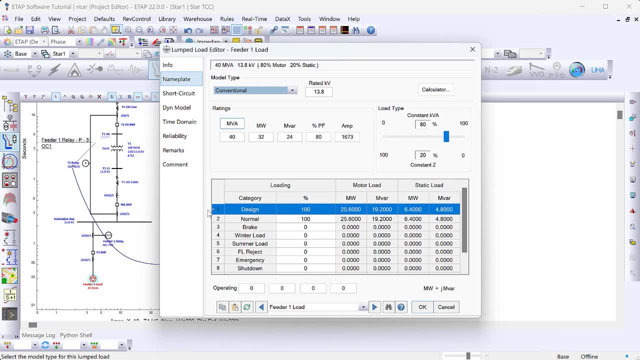 we can see that that's equal to 1673 amps and that's actually shown also over here on the load configuration. so again, 40 mba at our voltage of 13.8 kv is 16.73. so we're going to do something similar as to what we just did for the transformer. i can just take 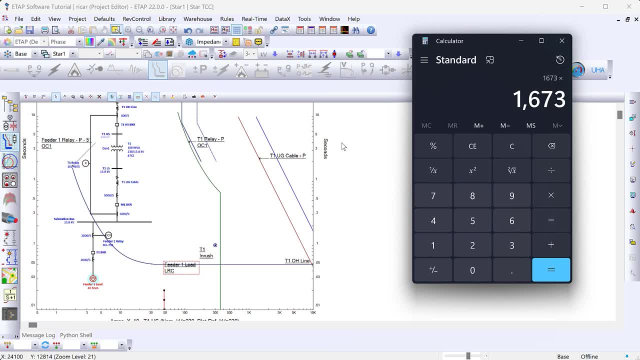 that number 1673, add margin to it. in this case i'm going to do 25 percent. so times 1.25, that gives us the worst case load current for our feeder, and then i need to convert that to secondary amps in terms of the real load. so i'm going to do that, and then we're going to do that, and then we're. 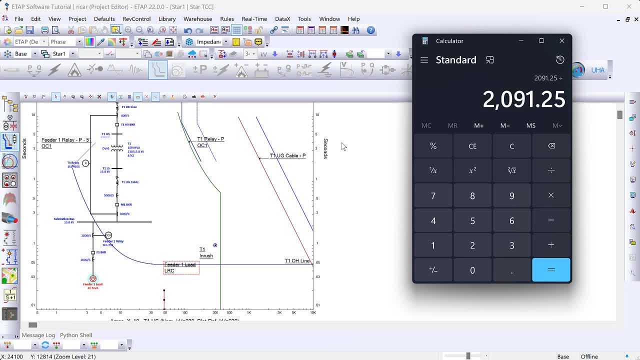 relay that is doing the protection. In this case it's this feeder relay which has a 2000 to 5 CT. So I'm going to divide this number by 400, which is 2000 divided by 5., And that's. 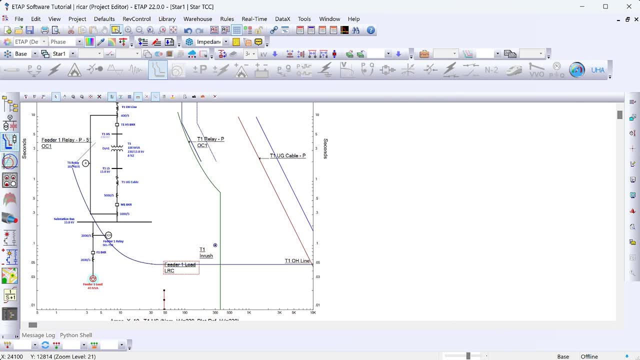 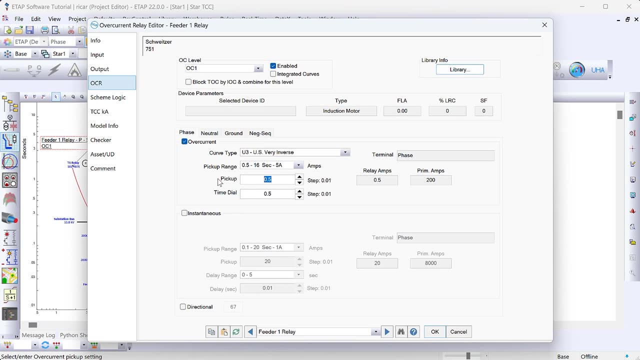 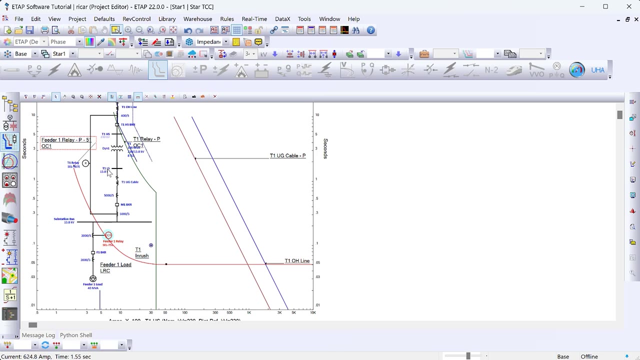 going to give me 5.23 amps for the pickup of this overcurrent element. So I'll sub click on this and I'm going to select this pickup to be 5.23.. And that, of course, moves our curve to the right. Now ATAP auto adjusted the view over here because it sees that now everything. 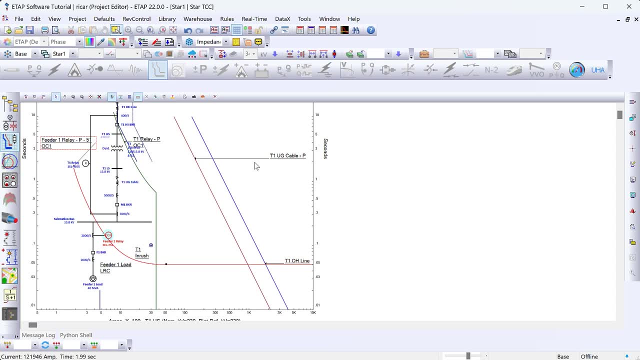 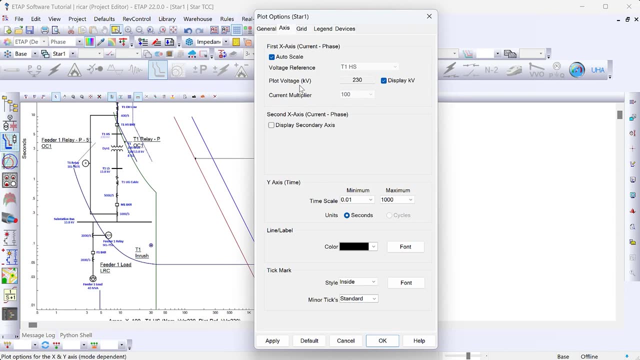 is kind of shifted to the side, So it changed the scaling over here. So let me actually double click over here So you can just double click on the background of the curve and go to access And you can see over here the auto scale and the current multiplier. Let me uncheck. 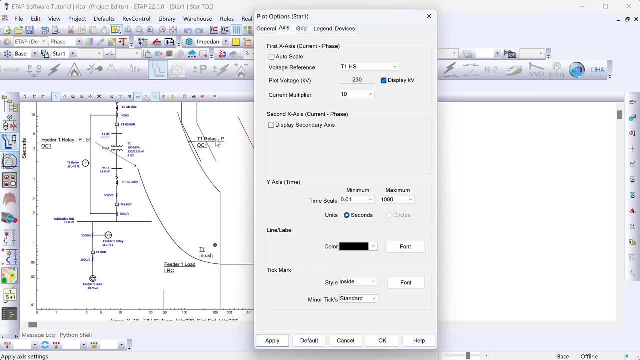 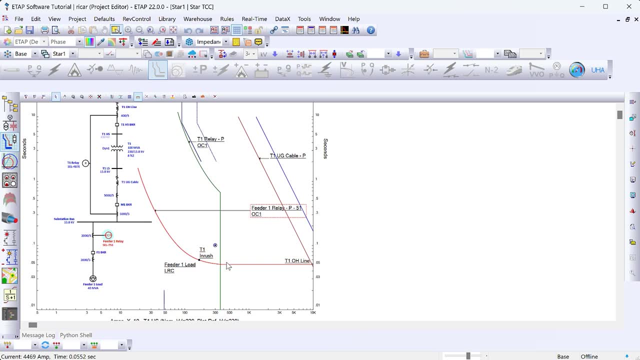 that and I'm going to move that to 10.. And you can see that that moved the curves over here to the right. I just want to do that so that it's a little bit easier to see the curves over here. Now you can see that with the default time. 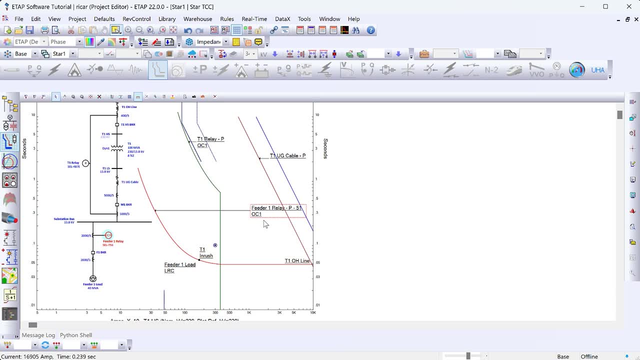 that I'm going to use. I'm going to use the default time that I'm going to use here, So that, of course, that's way down over here. I don't want that. What I want is to make sure that I have at least 0.3 seconds of coordination with this curve over here. Now to do that. 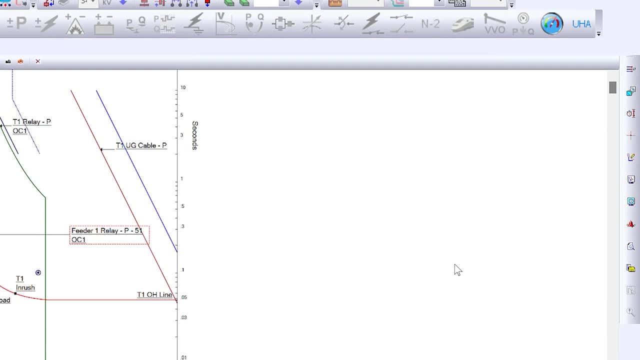 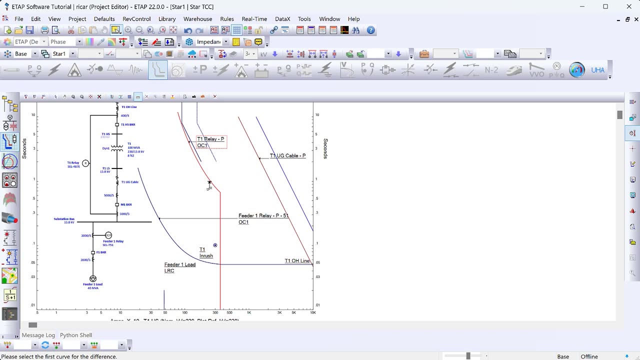 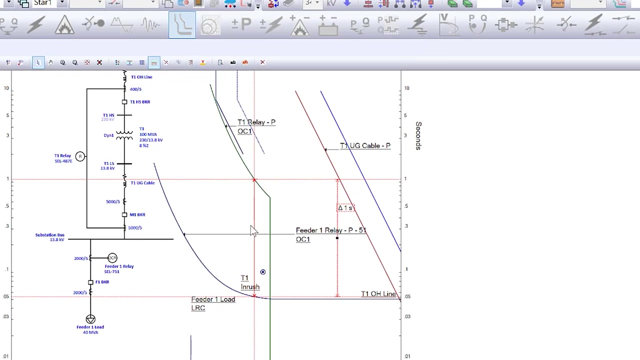 you can select this tool over here which gives you the time difference, And then you can click on the curves that you want to show the difference between. So I'm going to click on this curve Now. click on this curve and you can see that it put this marker over here. 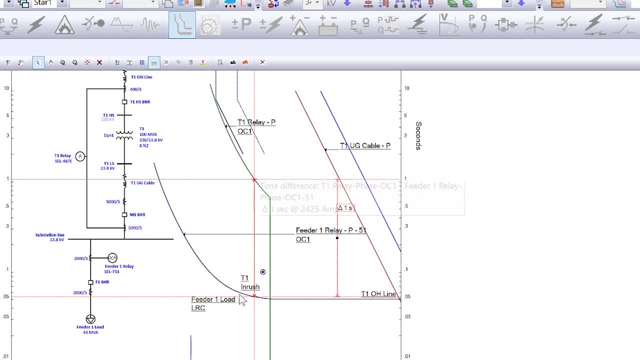 telling me what the difference is between this point and this point. It displays that over here It's saying that it's one second. Now, this cursor over here is actually just for display. This one here on the left is at which point on the curve we're coordinating. 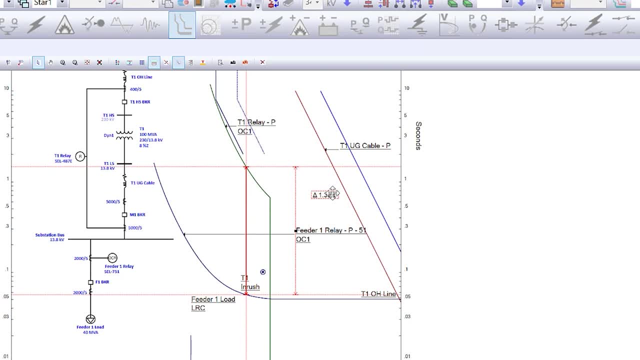 at. So, for example, if I move this to the left, you can see that this number changes to be bigger, because of course, the difference between this curve and this curve gets bigger. If I move it over here, that number gets smaller. So what I want to do here is basically: I want 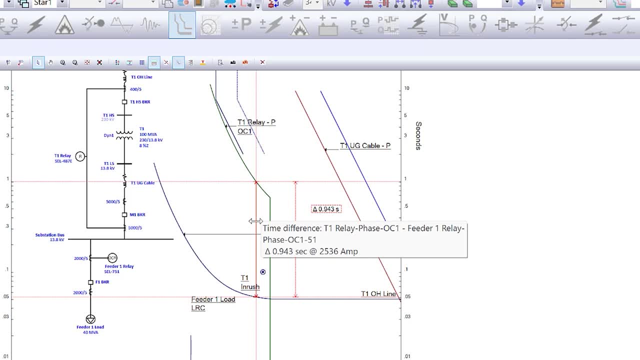 to coordinate these two curves at the worst case point. In this case, that's going to be right before that instantaneous picks up. So over here And now, I know that the difference between these two points is 0.64 seconds, And now I can click on my feeder curve and 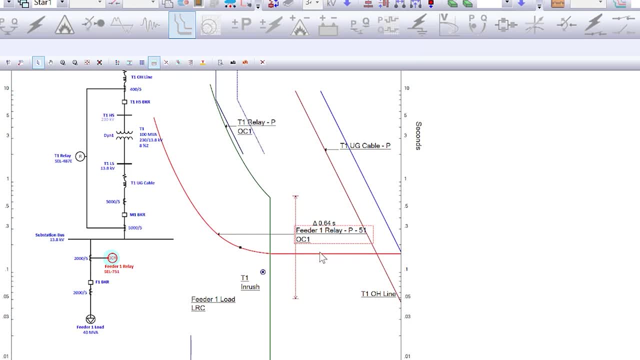 just drag that up so that our difference is about 0.3 seconds And this actually is not auto-updated. Let me move that here And I just need to refresh that. So now we have a coordination time over here between these two curves of roughly 0.46 seconds. I want that to be a little bit tighter. I. 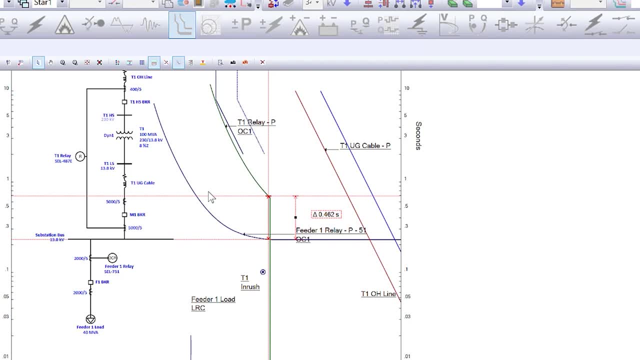 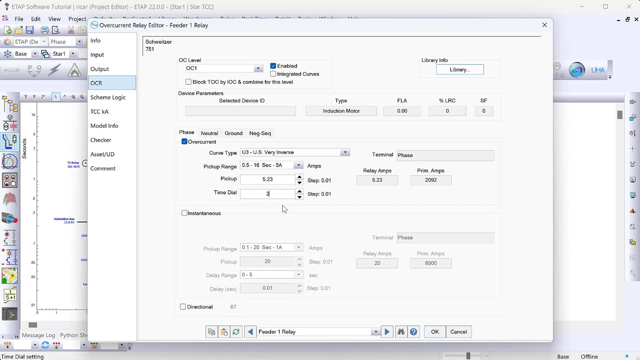 want that to be 0.3 seconds. So what I can do here again is I can either just click and drag over here, or I can change the time dial over here, And let's say, for example, that we have 3.6. Click, OK, And now you can see the difference between these two curves at. 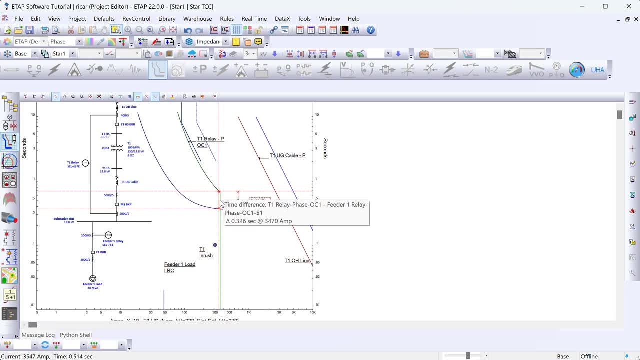 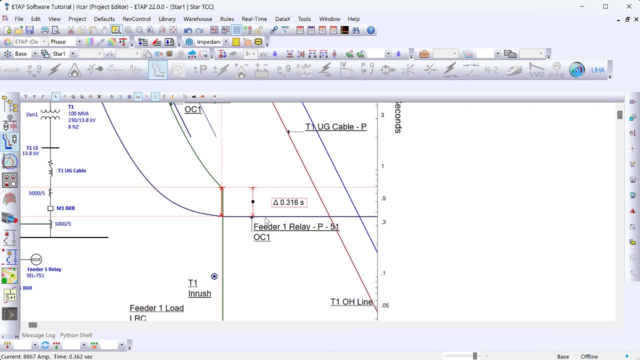 this point. over here It's 0.326.. So let me zoom in a little bit more and let's move that right before the instantaneous picks up. So over here that's roughly 0.3 seconds. That's the number I wanted. 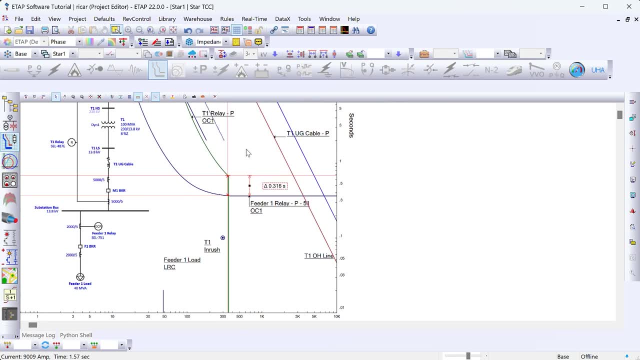 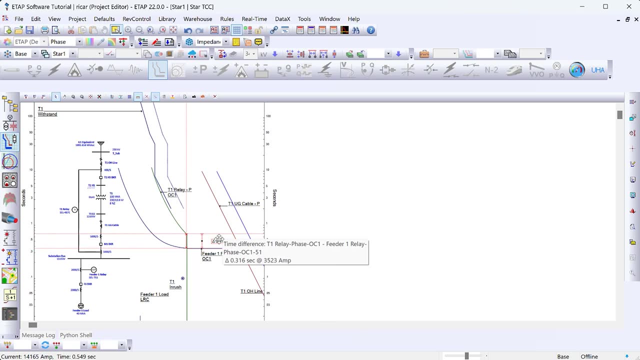 to see between my two curves. Basically, what this means is again the worst case. coordination time between the transformer curve and the feeder curve is 0.3 seconds, which of course, is over here at this point Now. lastly, of course you want to make sure that 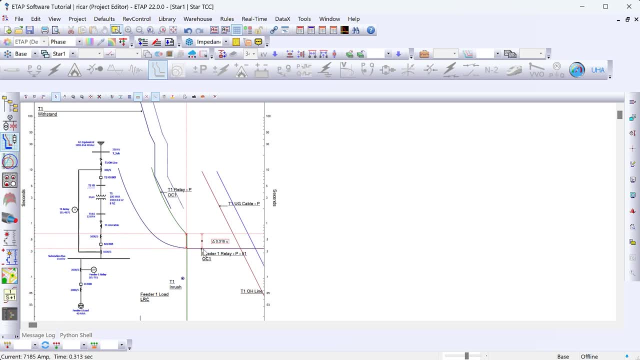 your curves are displayed organized. So what I like to do over here is: one: move this to the left such that it lines up with the other cursor, And then I also want to make sure that my settings are displayed. So I'm going to move just all these labels over here And 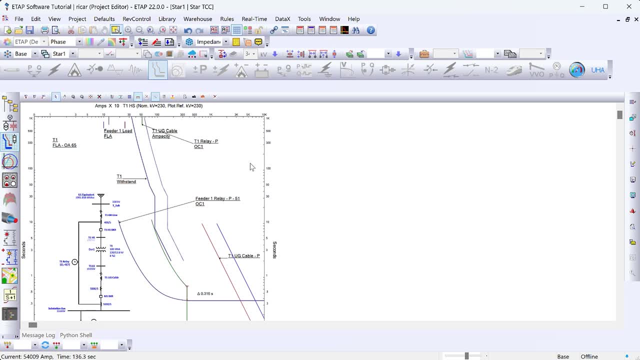 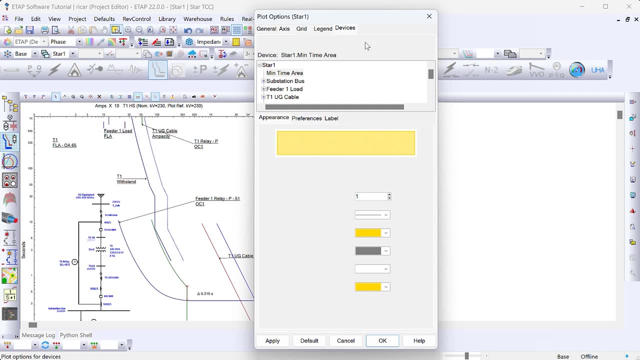 one thing that you can do over here is you can select what information to display. So you can double click on the background of the curve That's going to bring up this view, And I can see here over here two devices. This is the T1 Relay, which is the T1 Relay, and the Feeder 1 Relay. So if I go over here, 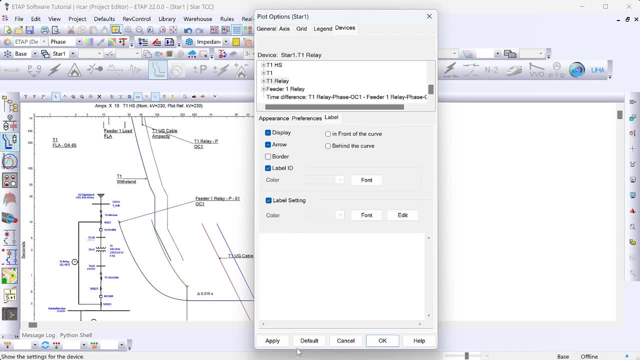 to T1 Relay, go to label label setting, hit apply And now that displays the settings over here. And I'm going to do the same thing for the Feeder Relay. Let's go over here to Feeder 1 Relay, So this one over here, go to the label tab and then click on label setting. 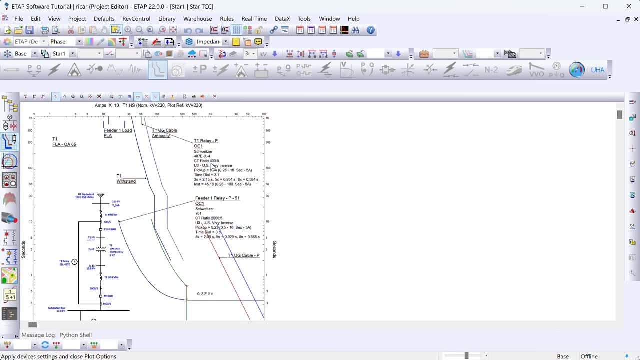 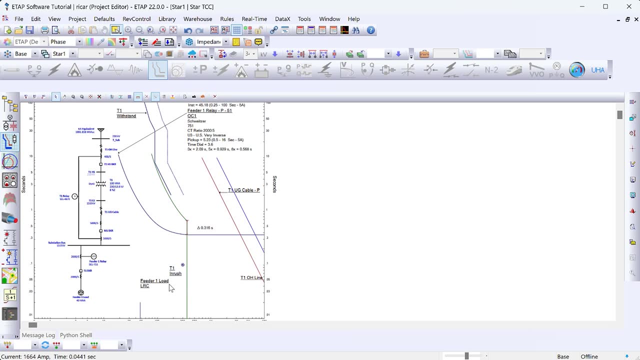 hit apply And again that displays the settings down here. So this is just a nice way for you to see the settings that you've applied on the same curve. you can also do the same thing for, for example, the inrush point over here. you can tell it. i want to show the current. 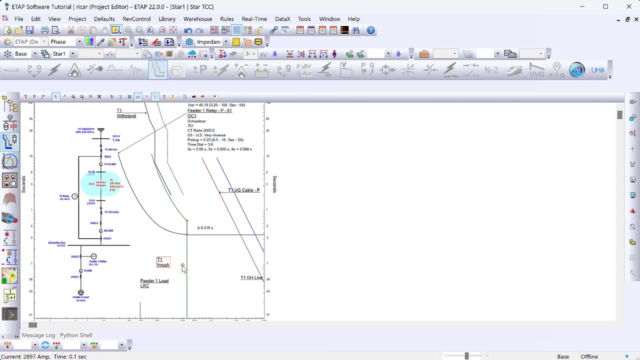 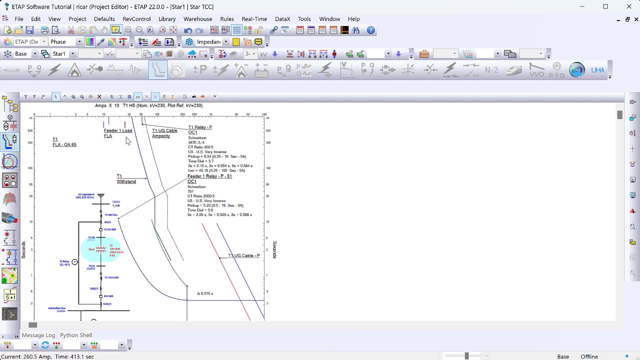 down here the current value. basically, what point is this on the curve? and again, typically i just try to clean this up a little bit more, just to make it a little bit easier to read. display this: maybe get rid of some of these curves over here that it's not really necessary for you to display. 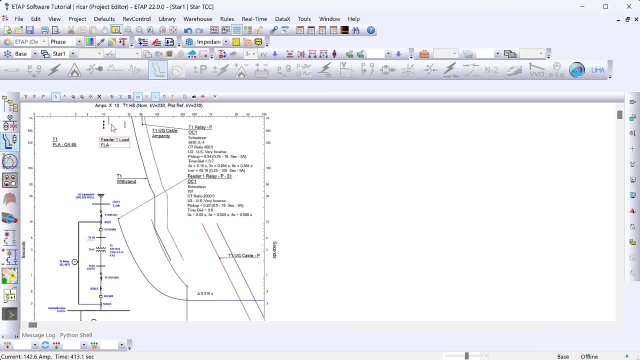 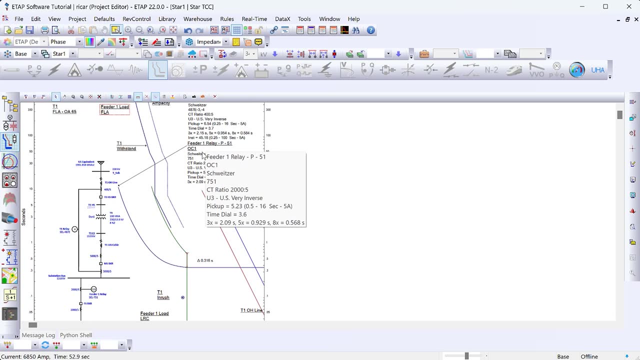 for example, the full load amps of the feeder load. typically i'll remove that- the lock rotor current for the feeder load as well. you can select what information you want to show on your curve and that just depends on your application and just the information that you want to display. but here 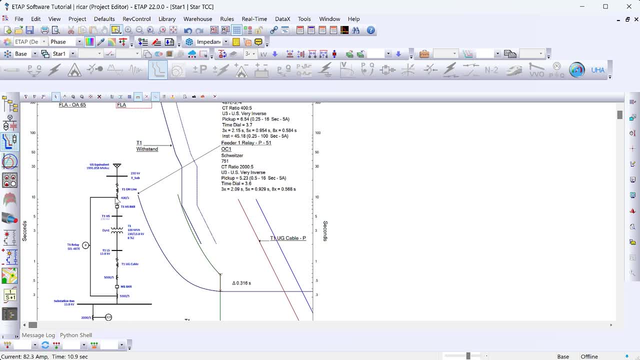 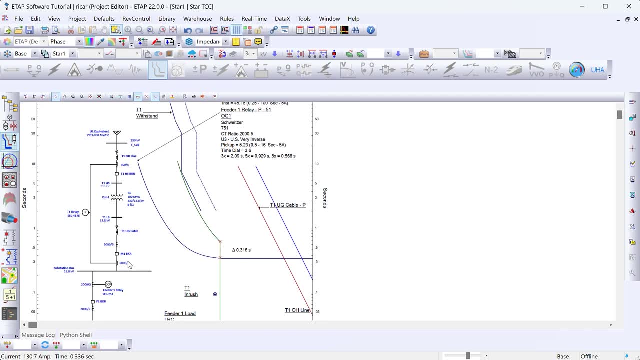 basically we coordinated the over current elements on the high side of the transformer with the feeder. we skipped the bus relay because we said, for this example, that doesn't have an over current element on it. but of course, if you had a relay here on the main breaker, for example, you would just do the. 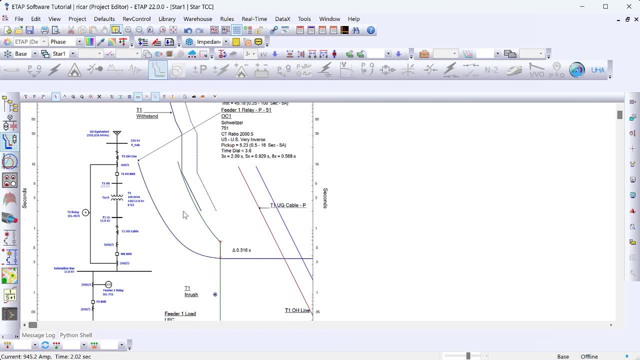 same process. you would have another curve here in between the high side over current and the feeder over current, and you would change the time dials such that you have at least 0.3 seconds of coordination between each one of the curves. so you would have a curve that looks like this, then another curve for the main breaker and this curve 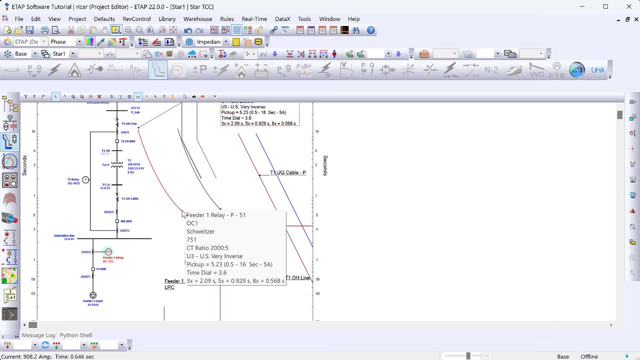 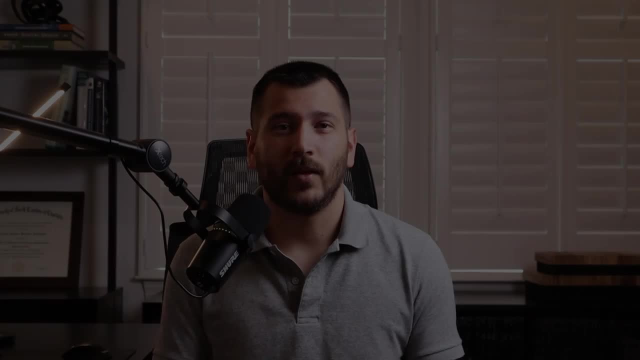 for the feeder would actually be a little bit further down, so that you have 0.3 seconds between the feeder and the main, and then the main and the high side over current on the high side of the transformer. all right, so that's how you run short circuit and protection coordination studies. 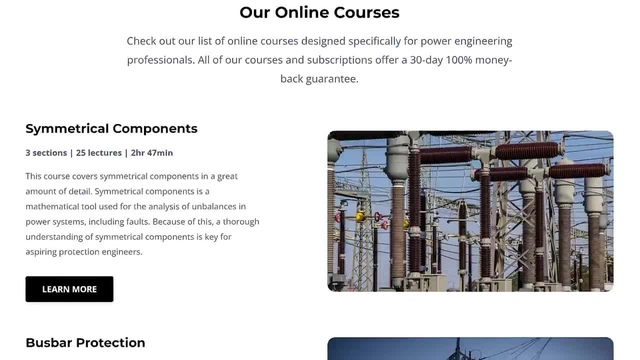 using the etap software. if you want to learn more about power system protection and control, make sure to check out our online courses, where we go over different types of protection schemes in a lot of detail. and, as always, if you like this video, make sure to hit the like. 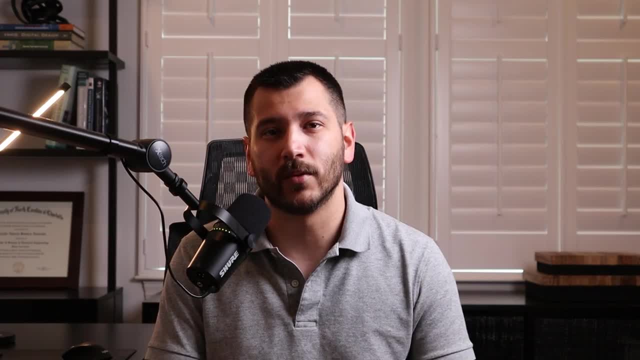 button and subscribe to the channel for more videos about power engineering and power system protection and control, and we'll see you in the next one.